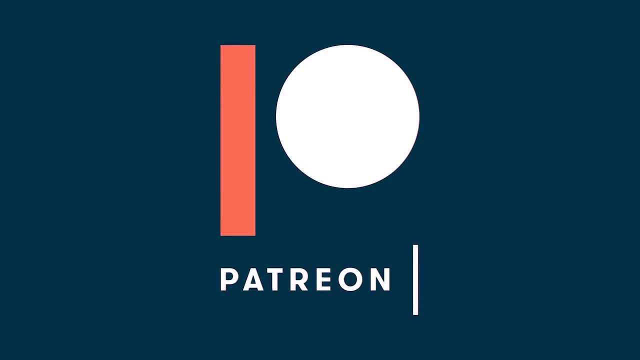 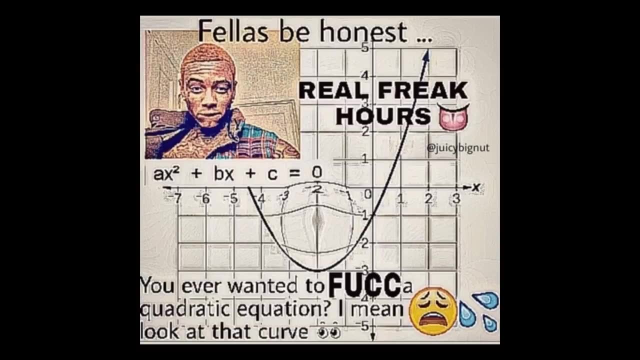 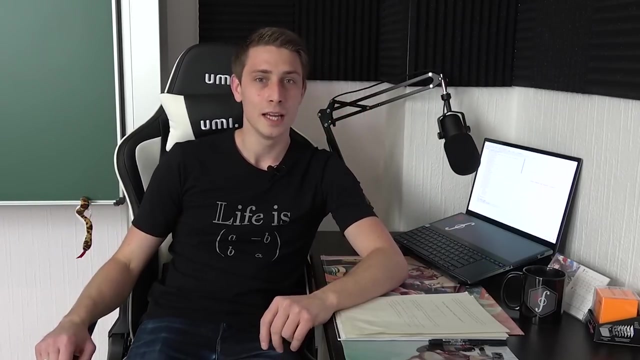 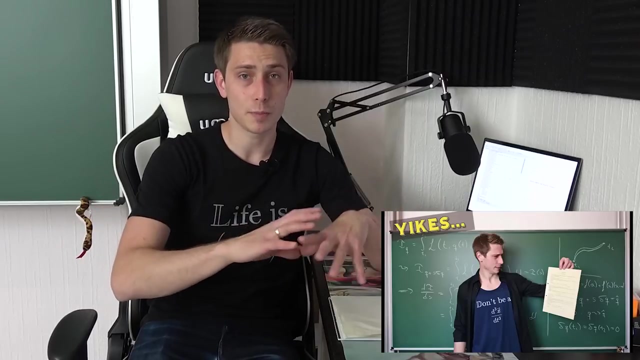 A huge thanks to my patreon supporters for making this episode possible. Good morning fellow mathematicians. welcome back to our video. First things first, all right. So if you are new here to the show, the hard exam playlist will be down there at the top of the description, Also the playlist where I work through a. 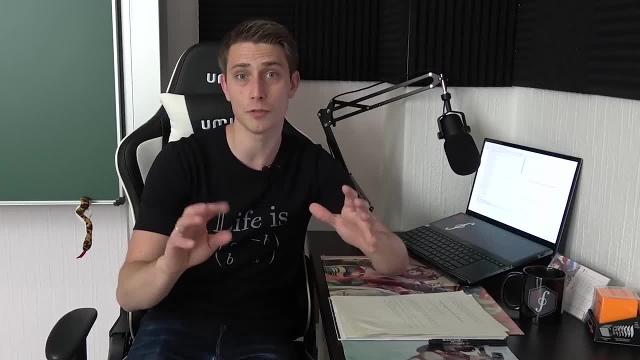 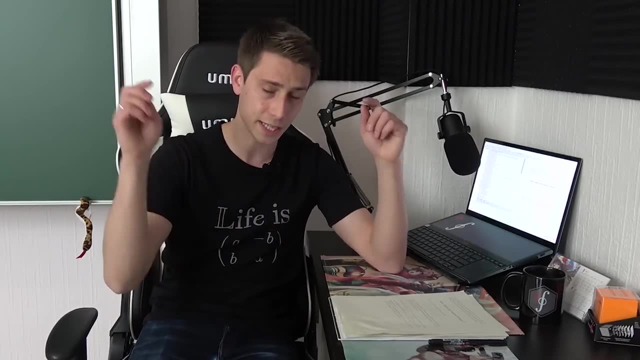 few of those hard exam problems. all right so where I solve them, and also, if you have any hard exams with a high failure rate that you want to send me that I should present on the show, then the link will be down there at the top of the description, the email address. All right, now for the main part. 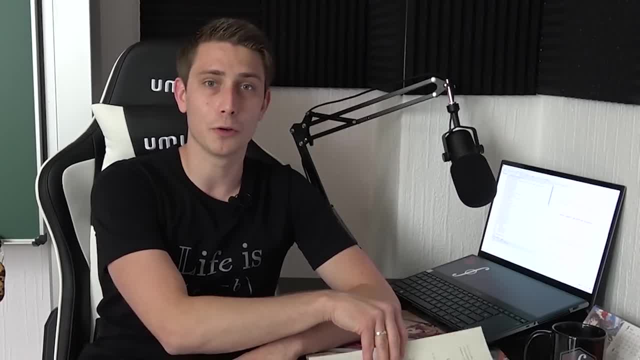 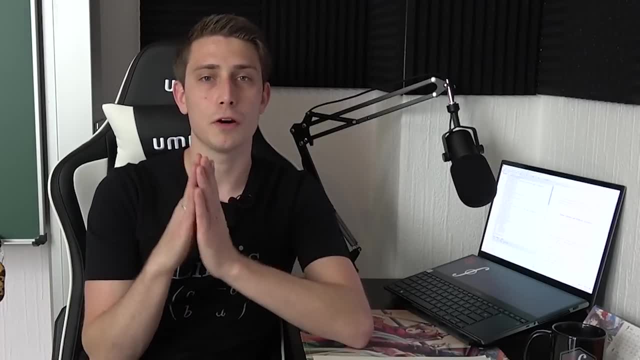 Hard exam series. yet again, We are going to talk about linear algebra and analytic geometry today, and here's the basic overview of what the video is going to be like. yet again, At first, some data about how many people participated, which semester, etc. 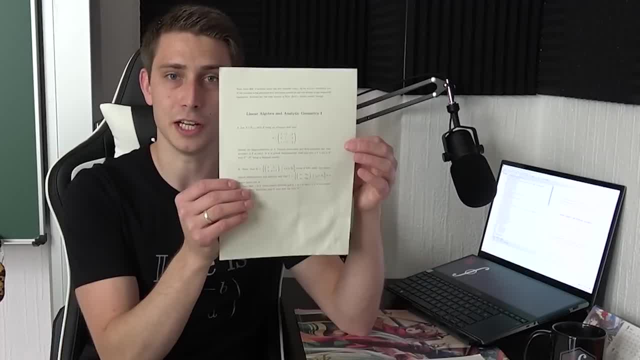 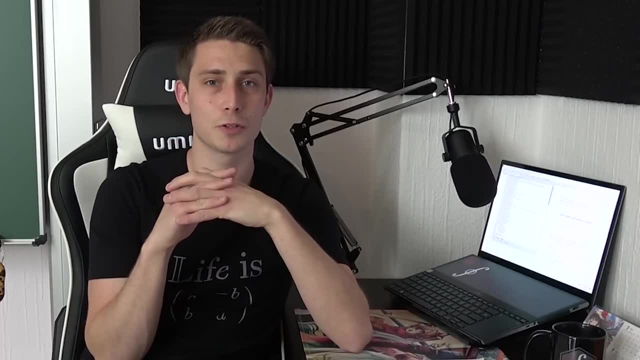 Then we are going to dive into the main thing, the linear algebra exam, And after that I'm going to tell you about a few reasons why so many people have failed in the first place, And I'm going to start this video off by reading what a 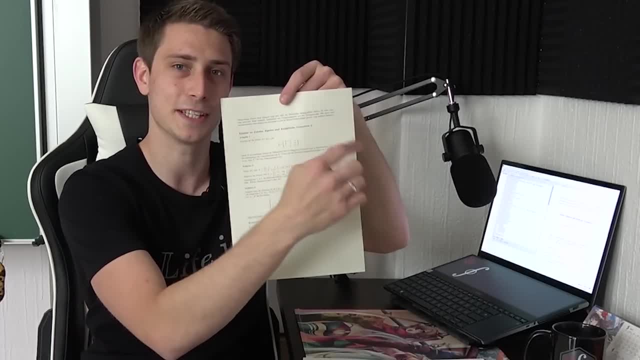 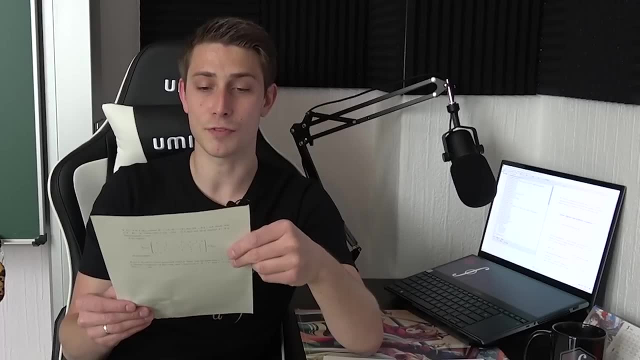 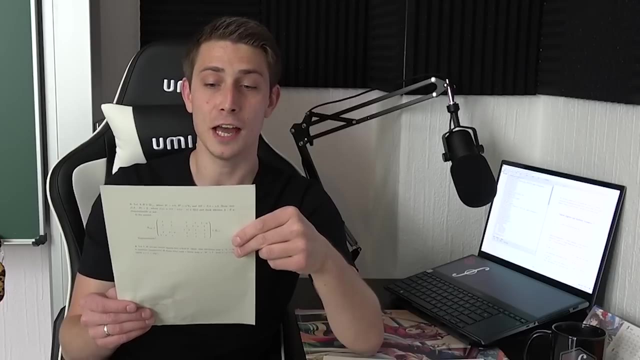 student has put up here on the copy of the exam. All right, I translated it into English. The person wrote over 90% of students failed this first semester exam. As far as I am concerned, none of the exercises being presented here have been covered in any way similar to any homework assignment. 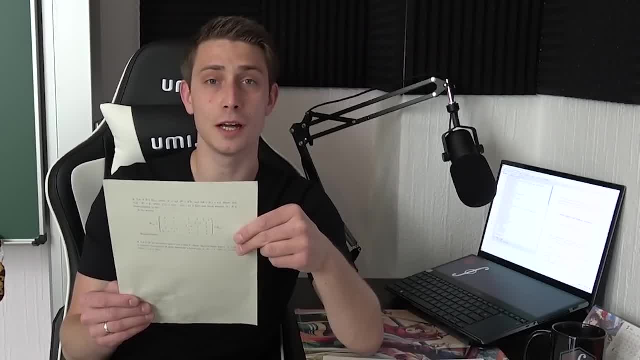 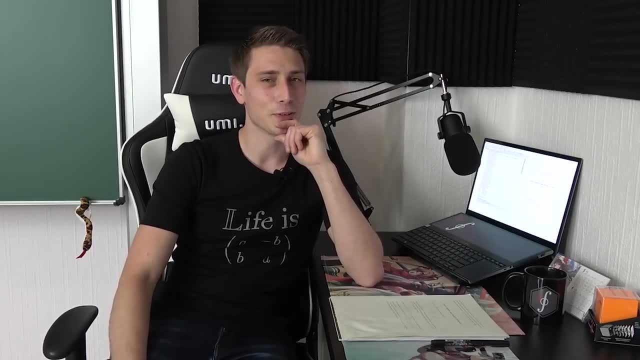 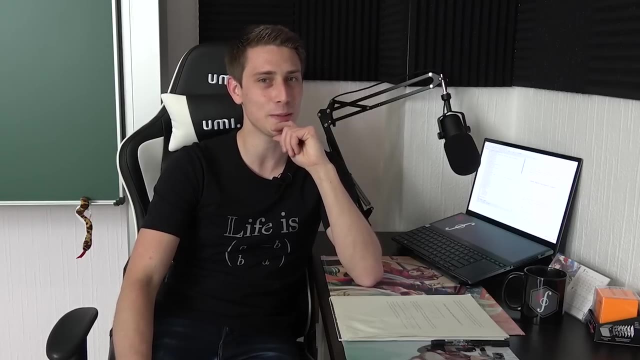 Exercise one has been covered in Professor Bras lecture or lecture notes partially, So now you have kind of an idea what's going on. All right, so the professor presented some stuff that maybe it wasn't really part of any kind of exercise. So no one was really prepared for that, And 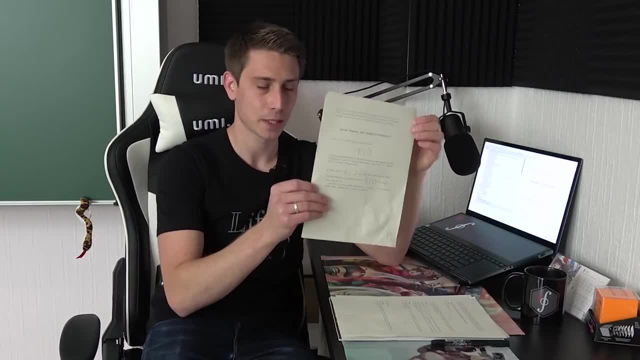 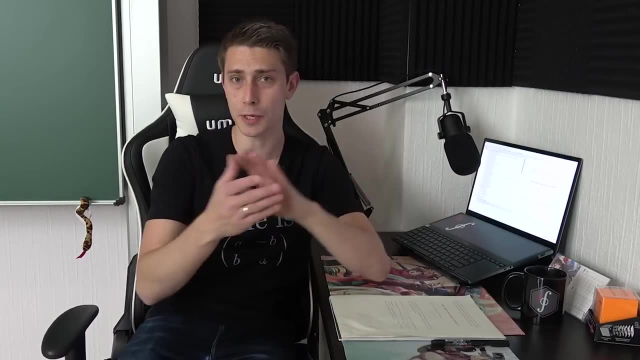 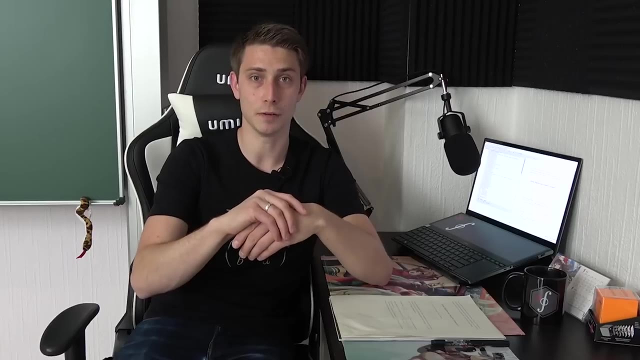 here's some data- First semester exam, So I can't really tell you how many people participated. I can only speak out of my own experience that about 200 to 250 people go into mathematics each and every year. So those are first semesters. They either become some kind of teacher, They are just there. 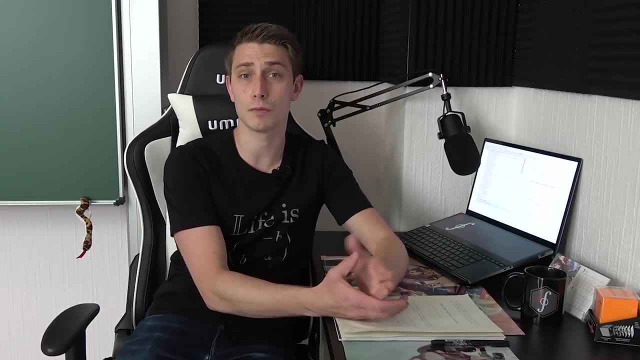 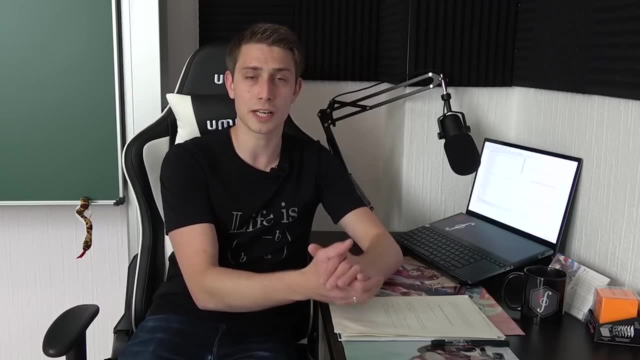 to be there just for fun in linear algebra, or they are going to become a pure mathematician or an applied mathematician in some way. So those are the kinds of people that are going to participate in this exam at the end of the first semester, And 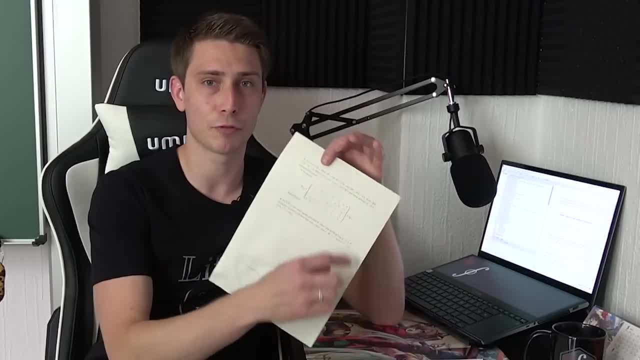 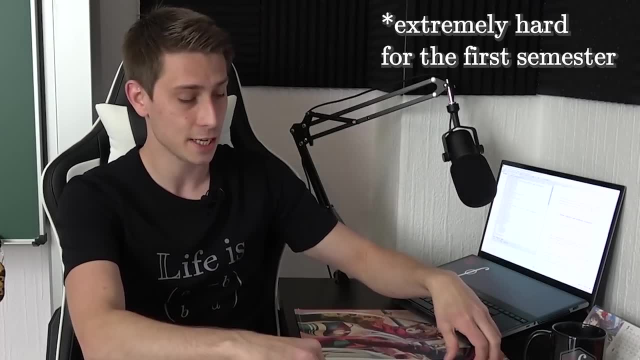 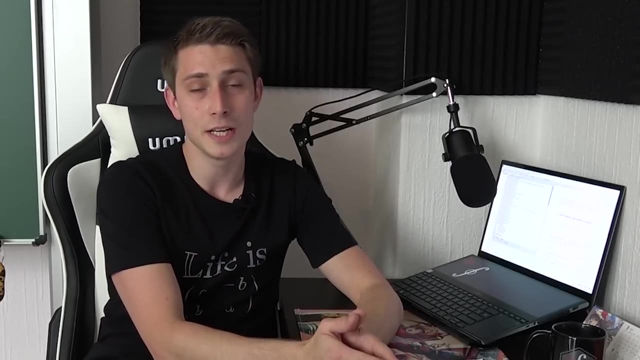 to be honest, this thing is kind of easy, except for the third exercise. This gives me terminal cancer. This exercise is extremely hard and it took me ages to get through this thing. So yeah, maybe it's just because I didn't know about some theorems whatsoever. It's just my opinion Also. 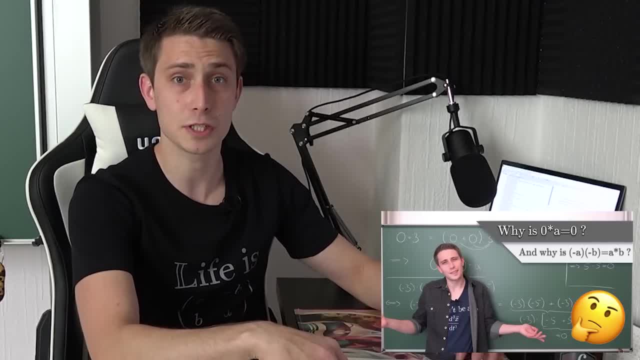 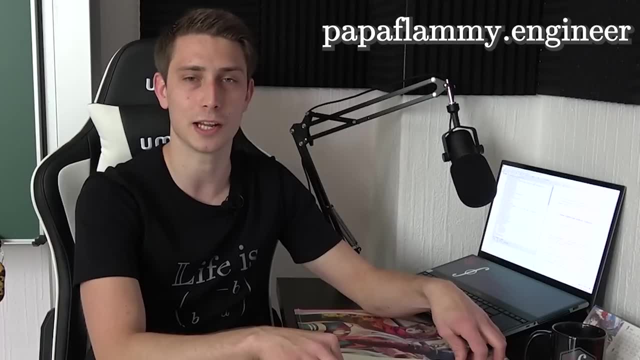 do not forget to check out my second channel. We just started a new series there. link will be at the top of the description. And also, don't forget to check out my new website. I made it with notion and I linked PapaFlammiengineer there. link will be also down there in the description. 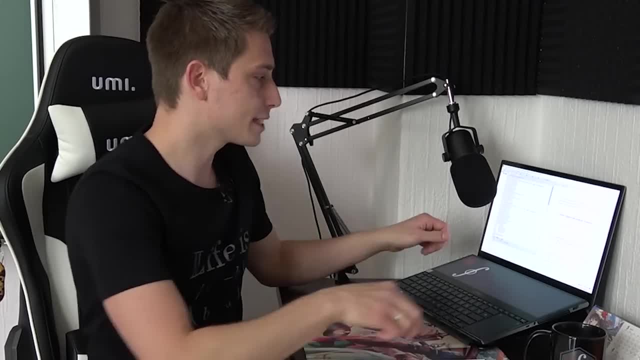 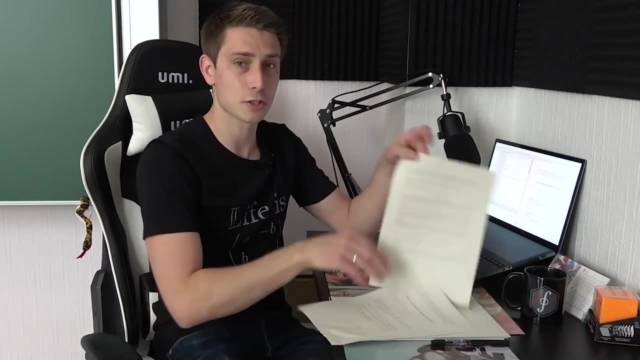 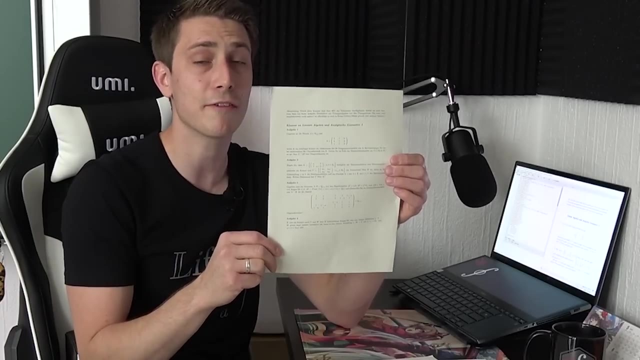 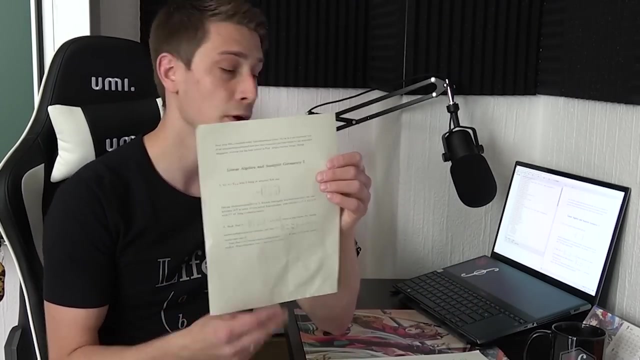 We are going to dive into this exam now. As always, I have translated the German version into English using LaTeX, So this is the original version: Four exercises: 12 points each exercise, 48 points in total. You need to get 50% of all the points to pass this exam. and here's the English version that I have translated for you: 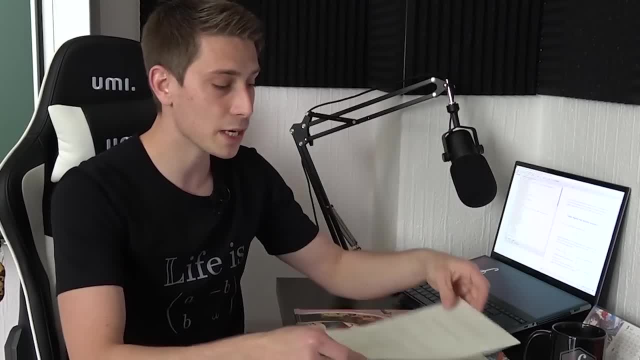 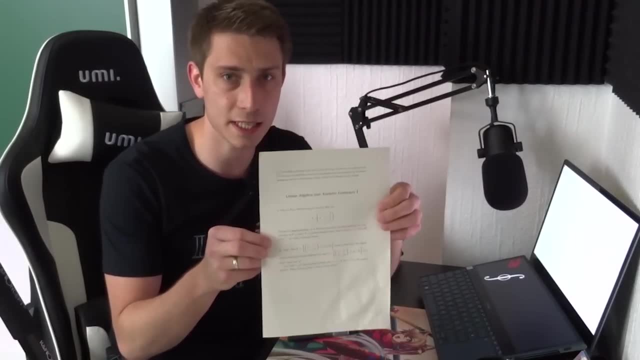 We're going to dive now into this exam and we are going to see what it actually looks like. All right, If you are wondering, by the way, This exam has been created by the same person who created the algebra and arithmetic exam, where 96% failed. 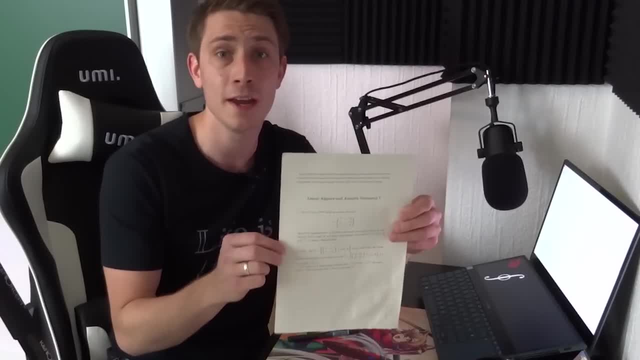 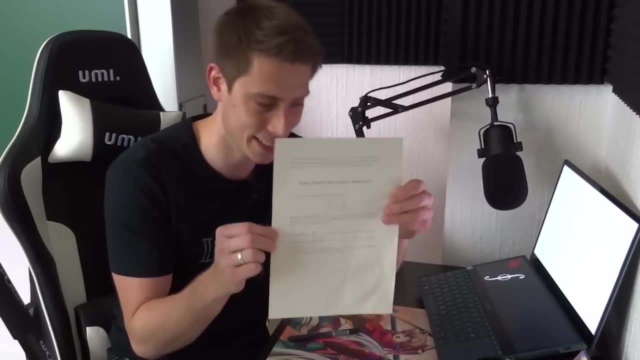 He's a substitute professor, sometimes for linear algebra. in the normal case He only does algebra and arithmetic, So now you know where he does come from. So he comes from field group and ring theory, and this is mostly the most hardcore thing at university for most undergrads. 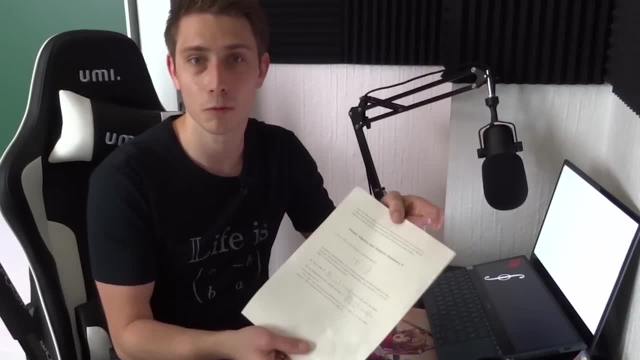 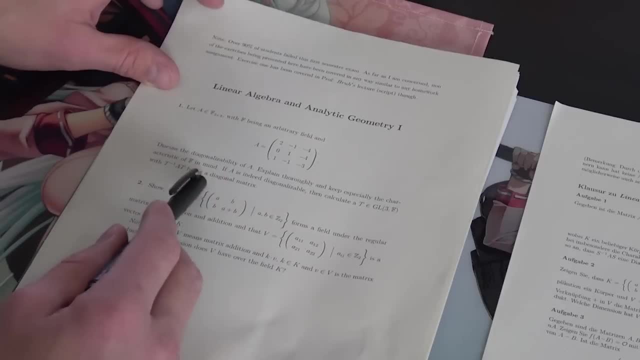 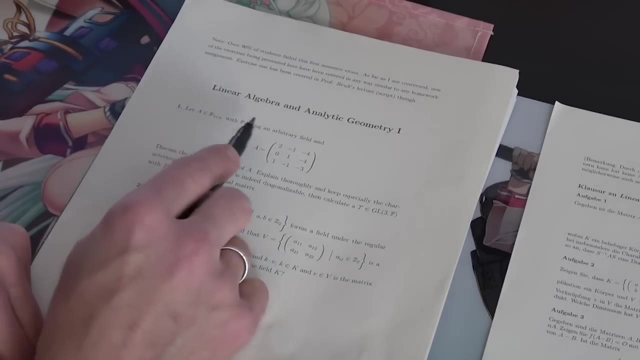 We're now going to dive in and we are going to see What's the big deal about this exam here. So, like I mentioned before, we have four exercises, Each with 12 points. you need 50% to pass this thing- And the first exercise Basically just deals with a 3x3 matrix in some random arbitrary field. 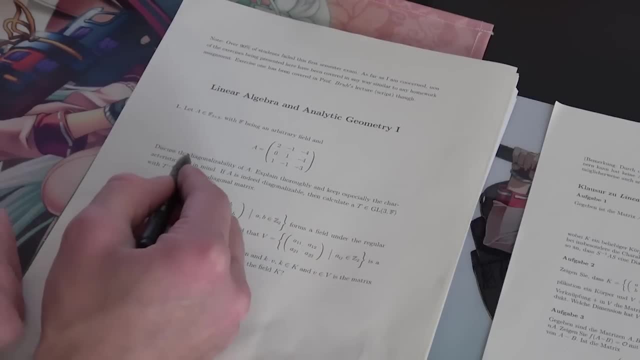 We are going to call it F and we want to discuss the diagonalizability. I have practiced this word so often in the last few days, such that I can say it nicely in this video. Just just listen to it: diagonalizability, Diagonalizability. All right, so we need to check for the diagonalizability. 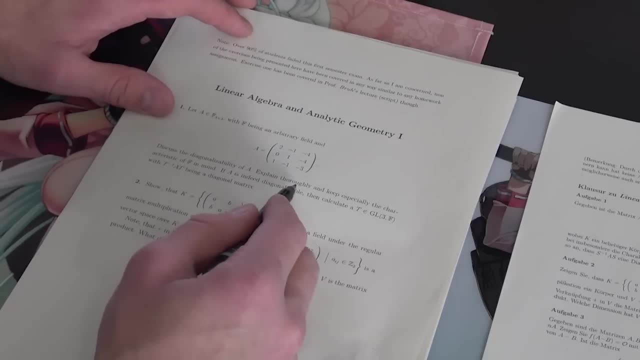 great pronunciation, papa of A, and we want to explain thoroughly- and Yeah, we want to explain thoroughly- why it is Diagonalizable. and also we wanna take a look at the characteristic of F, if there's something we need to take into account in order for it to be. 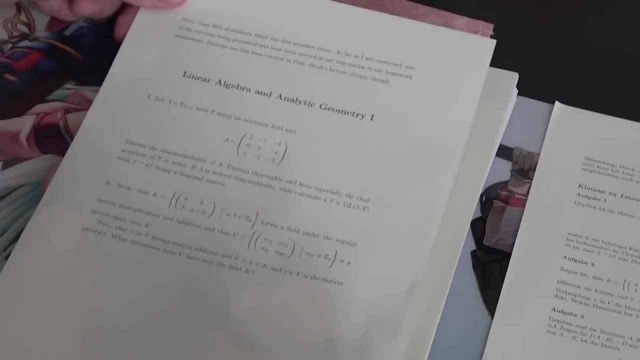 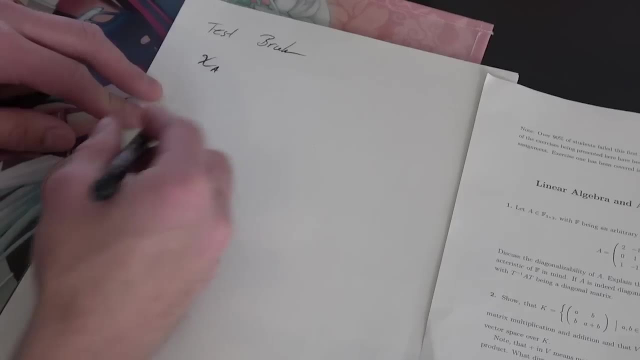 Diagonalizable. so here's the basic structure, what you need to do. So, at first, this was our matrix A, and we need to calculate the characteristic polynomial in some way of A, which is, nothing but, well, the determinant of A Minus. Well then we have our eigenvalues. that we don't know yet. we are going to get three eigenvalues. 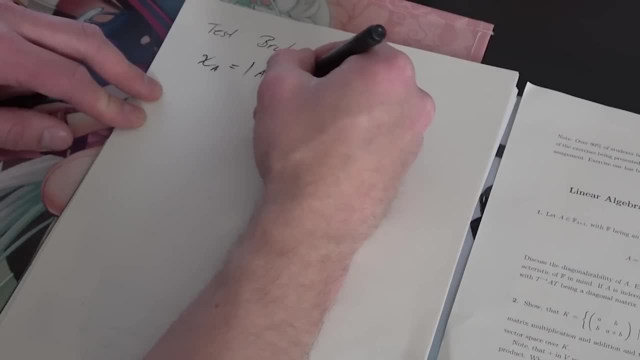 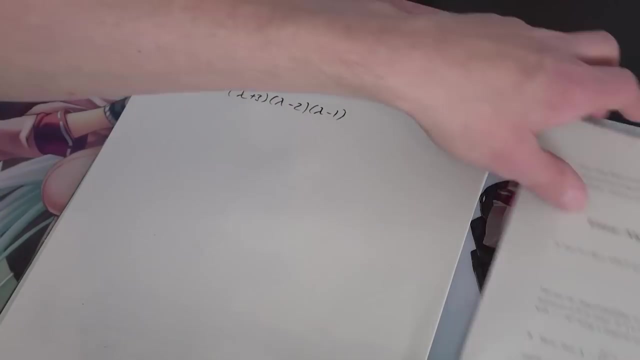 We don't know if they are common�, they are distinct. yet times the identity matrix in three dimensions and we need to set this equal to zero. After you get this whole polynomial, it should be something like lambda plus three times lambda minus two times lambda minus one. Good thing is: a lot of stuff cancels out. you can just. 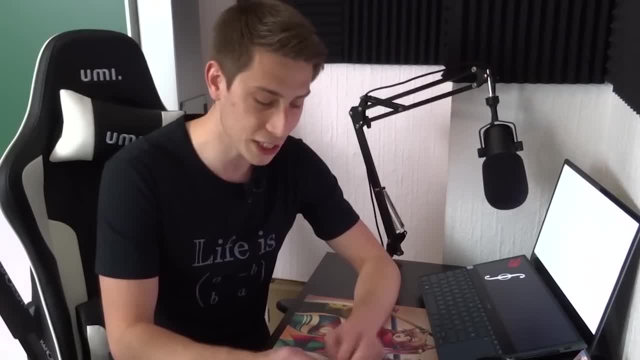 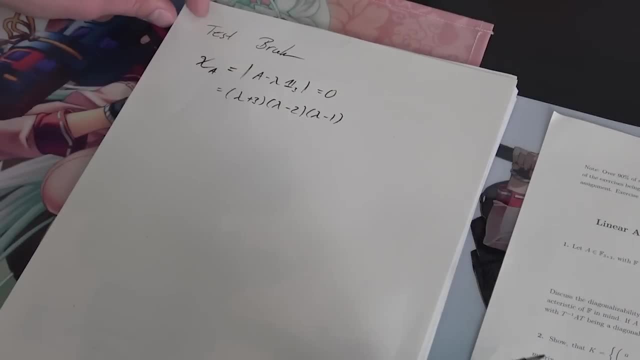 make use of sorry's rule here. I'm terribly sorry, and the eigenvalues are what you have here on the main diagonal basically. So those are the eigenvalues, and now we need to take a look at a characteristic, because it can happen that if you are in a field with characteristic two, 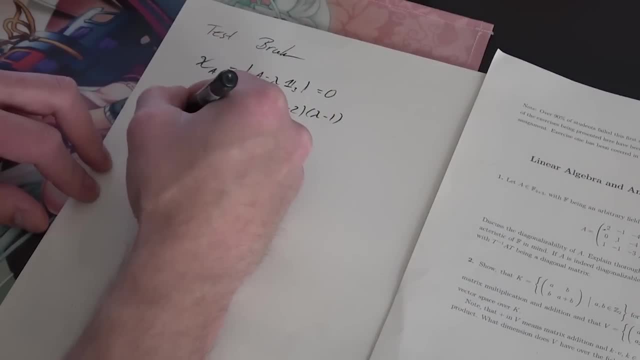 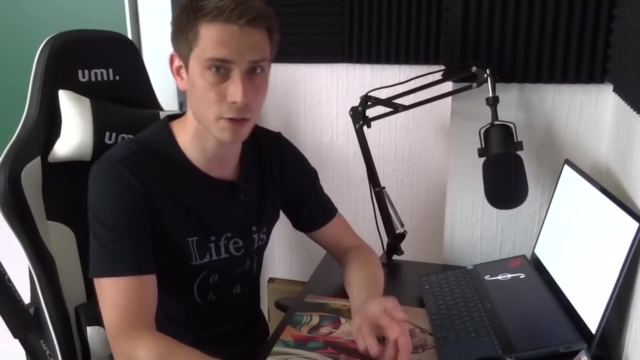 or three. so a field f can only be a field if the characteristic of it is prime. p is prime, all right, so this is what we need. two and three are prime, so we don't need to take a look at f1. this doesn't exist. okay, this is one of my deepest wishes: that f1 would be a field, but it. 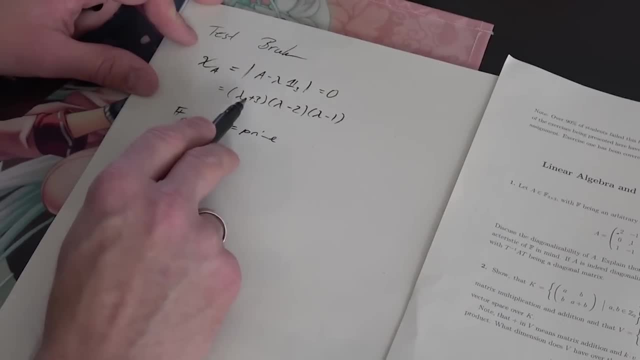 is not. So we need to take a look at f1. this doesn't exist. okay, this is one of my deepest wishes: that f1 would be a field, but it is not. isn't all right? so yeah, so we need to take a look at the cases where we have modular three. 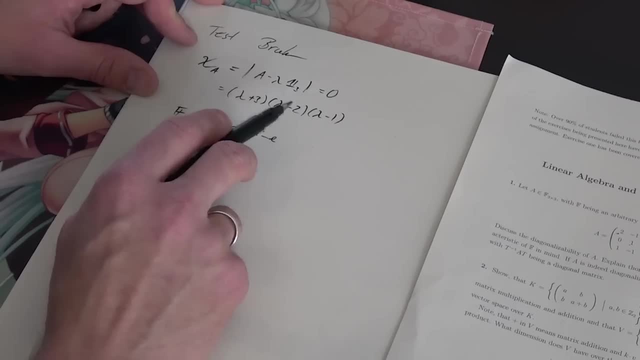 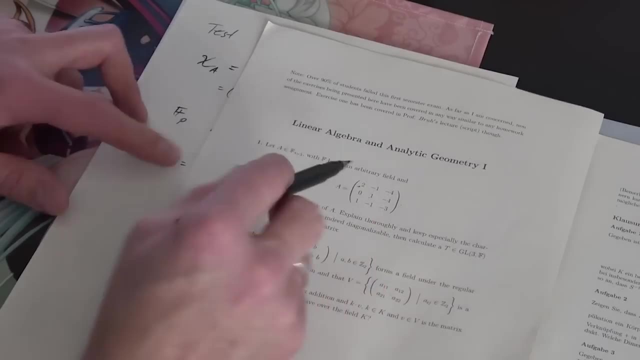 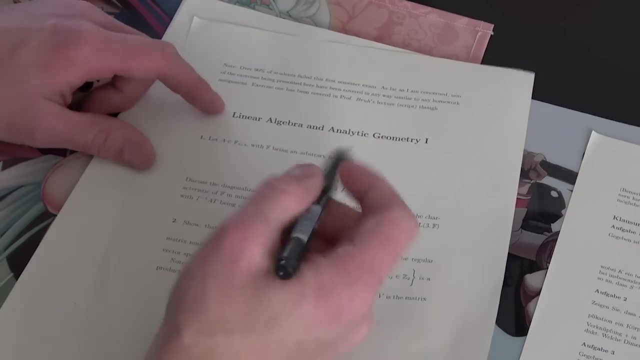 or where we have modular two corresponding to those eigenvalues. if we are in f2, then, for example, a is going to look like this: a in f2 is going to be all right. so two, so all multiples of two, are going to be zero. this gives us zero, and then negative one is exactly one in modular two. yet 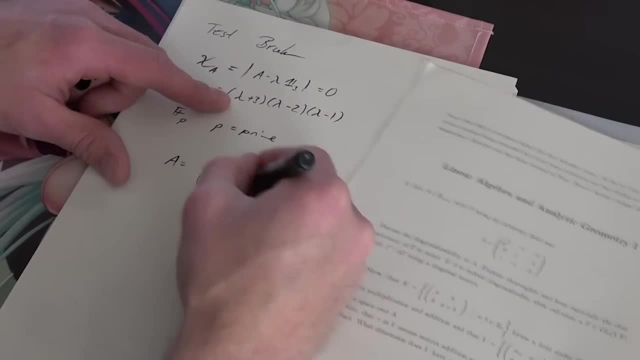 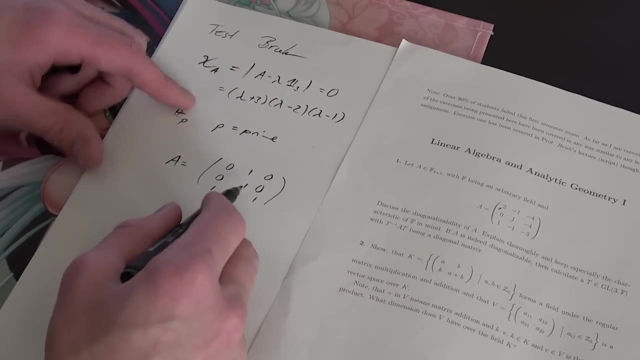 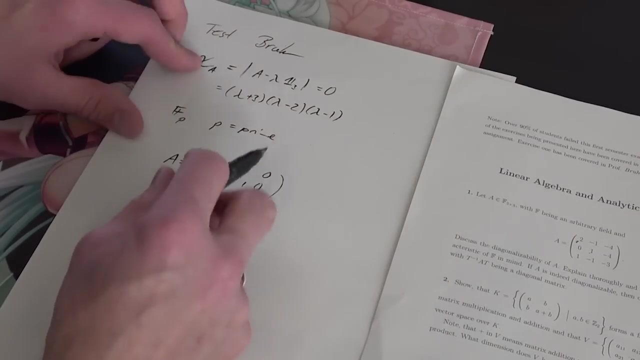 again. so zero one, zero. then we have zero, one zero, and then one one and negative three is exactly one. yet again, this is what it looks like in modular two and, yeah, this thing is actually not diagonalizable if you check for everything. this just has to do with the um, with the eigenvalues that we are going to get out of it. 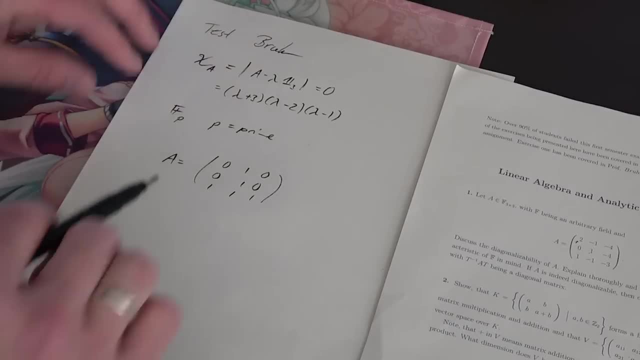 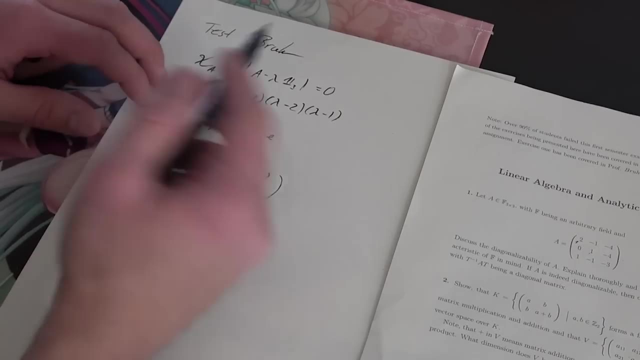 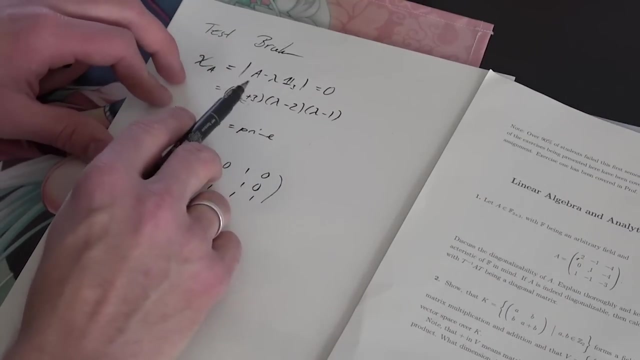 and it just doesn't happen. it's just not um diagonalizable, because three in modular two would be one yet again, and it just doesn't work out. so the geometric multiplicity isn't equal to the algebraic multiplicity in this case. so for f, f2, it doesn't work. for f3 it should work out. in my opinion, it should work out. 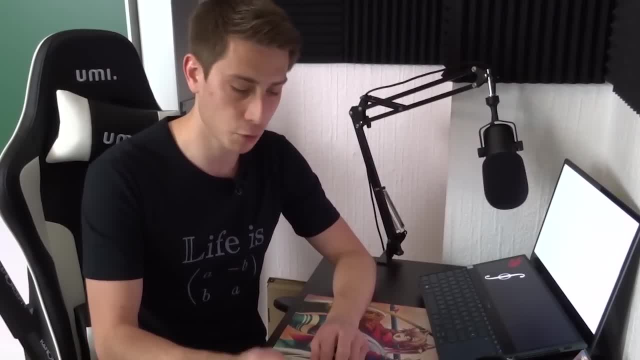 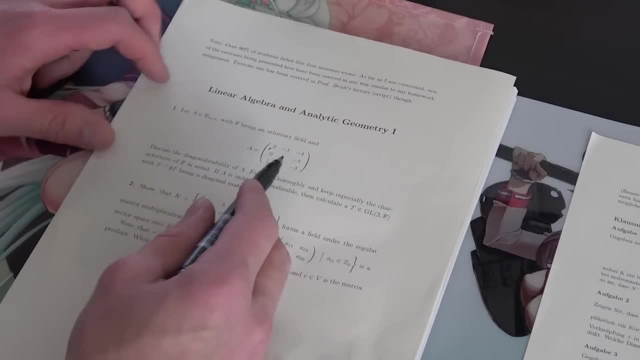 correct me if i'm wrong on this one. so this is all you really need to do for this. otherwise, in each and every other field it's just going to be like diagonalizable. you just check for um the dimensions of the eigen space and the corresponding eigenvalues with algebraic multiplicity of one. then 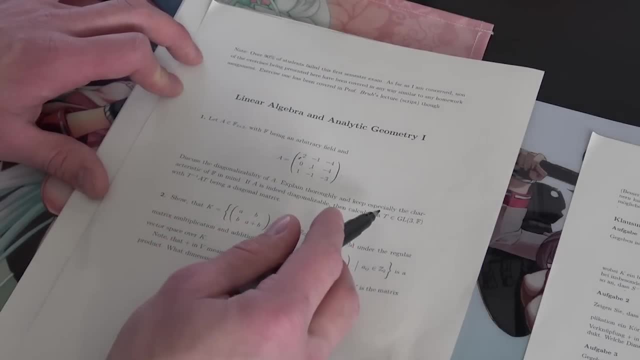 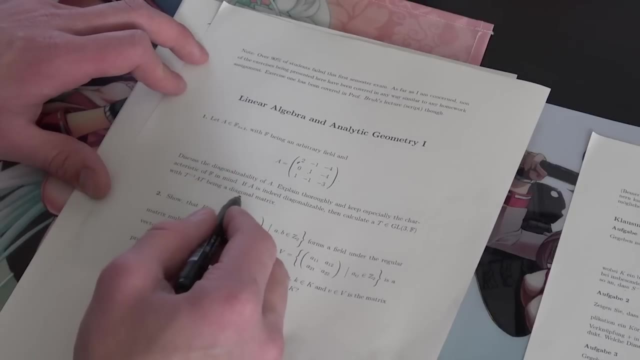 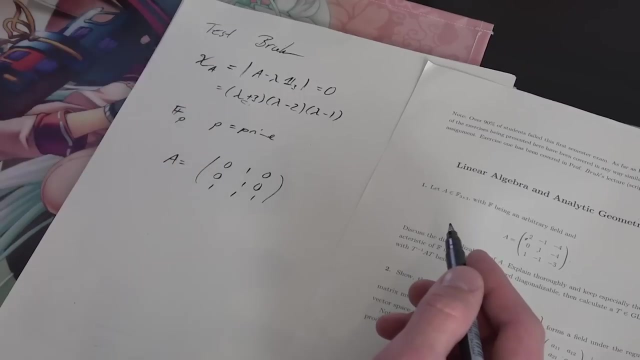 if a is indeed diagonalizable, then calculate a t element of gl three in this field. f with t to negative one times a times t is a diagonal matrix, all right. so yeah, calculating this t is just a straightforward process. you just need to find one that does it. 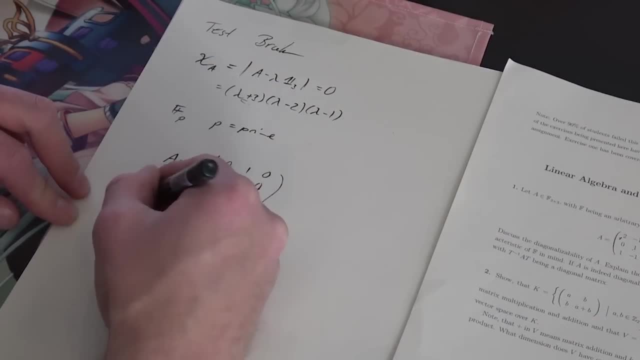 and then you are just going to go through this whole thing. you are going to take a minus. the first eigenvalue, for example, times the identity matrix, three dimensions, times some vector- x, y, z- is equal to zero vector. so we want to find out the kernel, so the homogeneous. 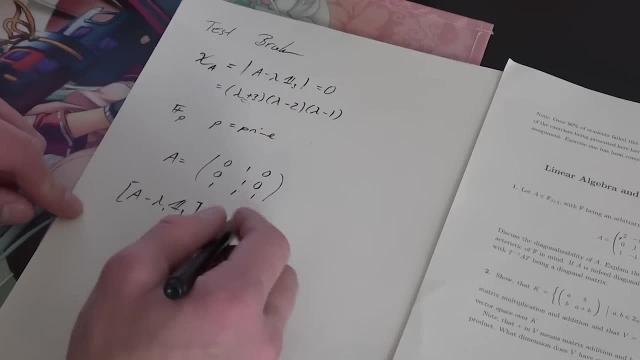 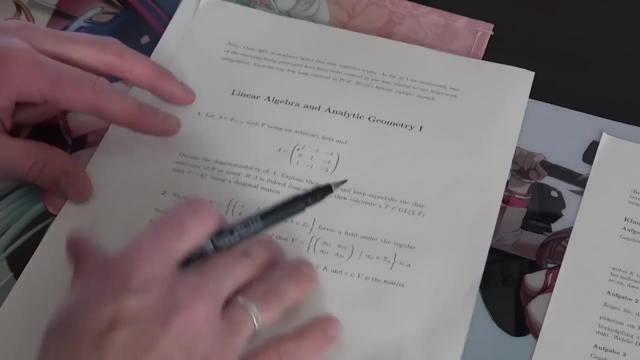 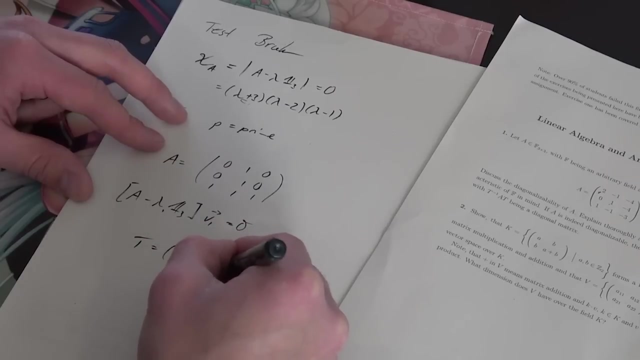 solution for each and every eigenvector. this is just the property of eigenvectors. you are going to do this three times overall, and after that you are basically done with this. you can find yourself a t where, so this is the vector v1, and then our t is nothing but v 1, v2 and v3. okay, 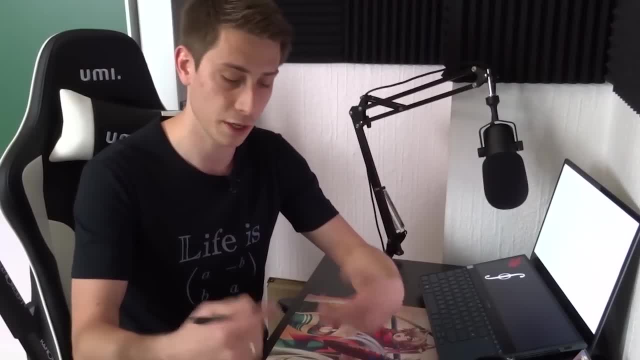 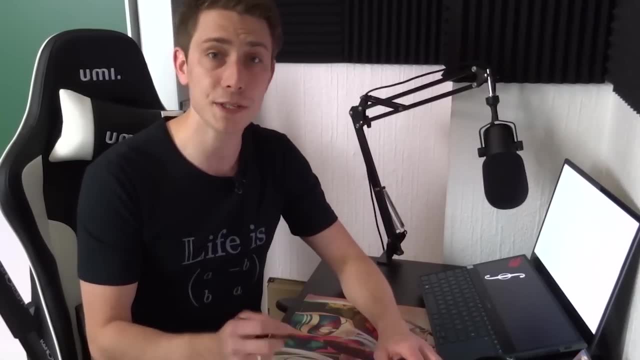 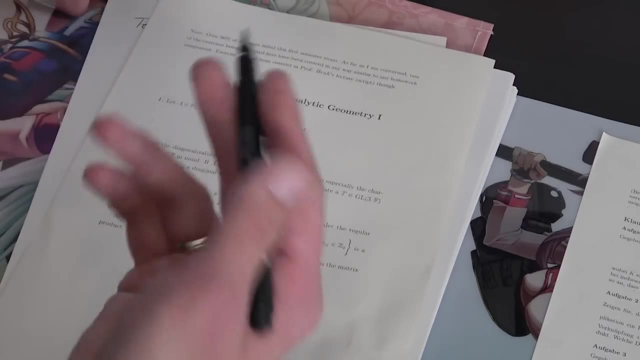 that's going to be our matrix. then you can invert it, check for invertibility and then you are basically done. that was the first exercise- really easy. first exercise is really easy. same spiel for the second exercise. show that k forms a field under the regular matrix, multiplication and addition. you just go through the field. axioms means. 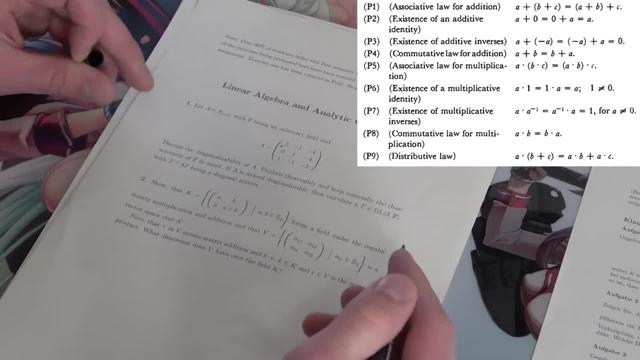 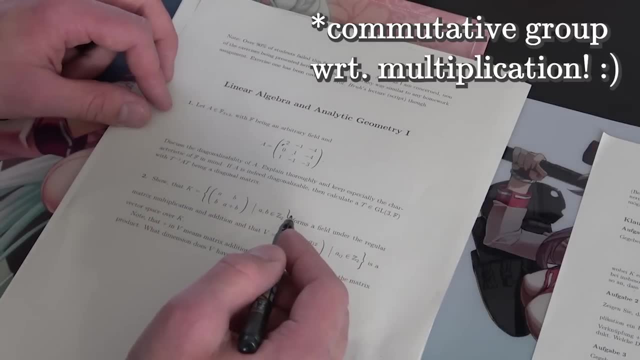 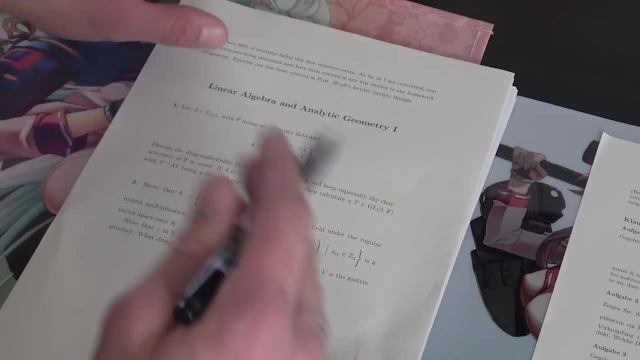 distributive laws, then we need a commutative group with respect to plus and we need a group with respect to times. all right, so yeah, and this group with respect to the multiplication is just going to be without the zero matrix in there. so does work out. you just go through all those axioms. 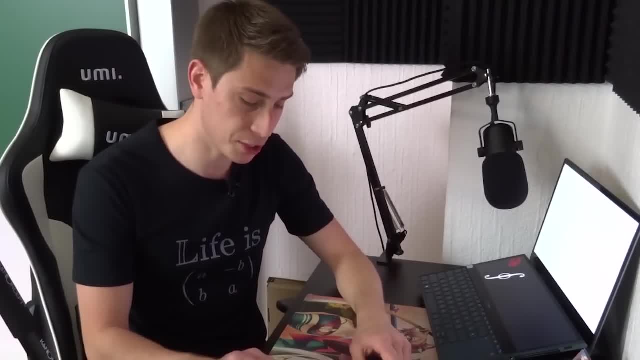 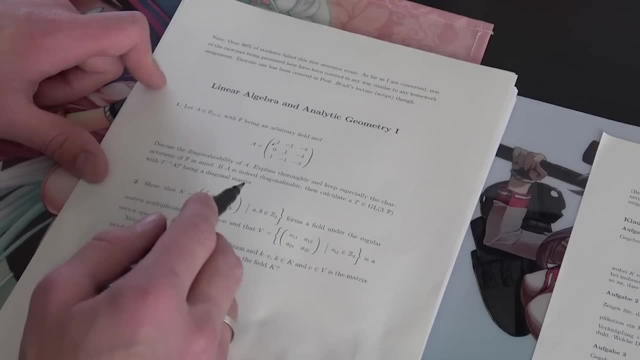 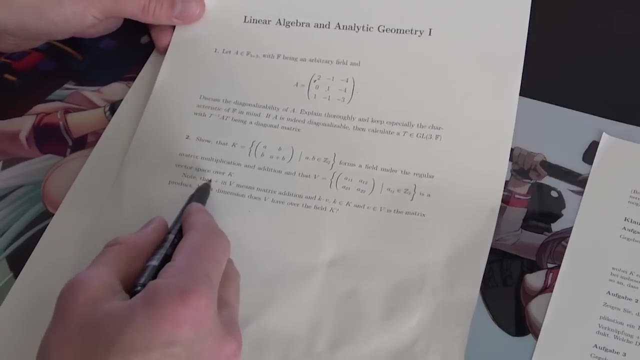 it's going to be really easy. next up is a bit more work. we need to show that a v being defined like this is a vector space over k- yeah, over this field k that we have here. it's really easy to show. just go through the vector space axioms, it's really easy. then note that plus and v means 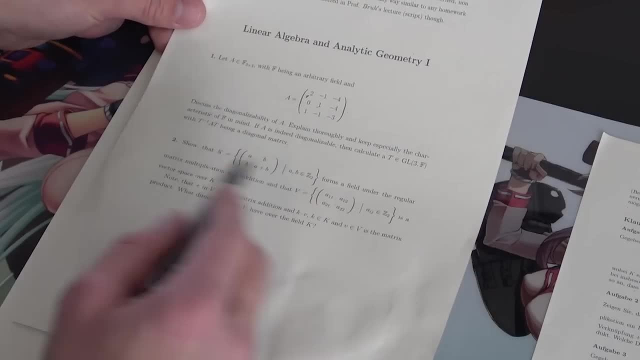 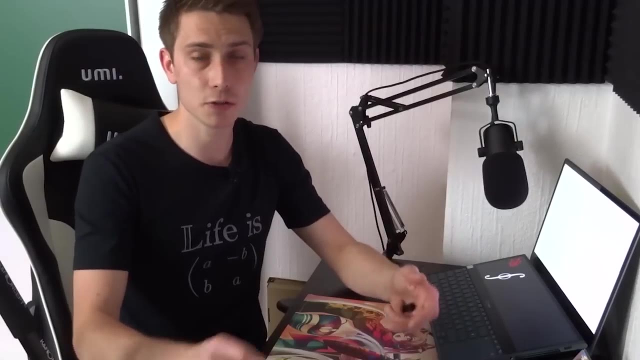 matrix addition and k times v is just a scalar multiplication. we know this. so matrix, matrix addition and k times v is just a scalar multiplication. we know this. so matrix addition: matrix addition and k times v is just a scalar multiplication. we know this. so matrix addition product. and what dimension does v have over the field k? you can use some dimension theorem or 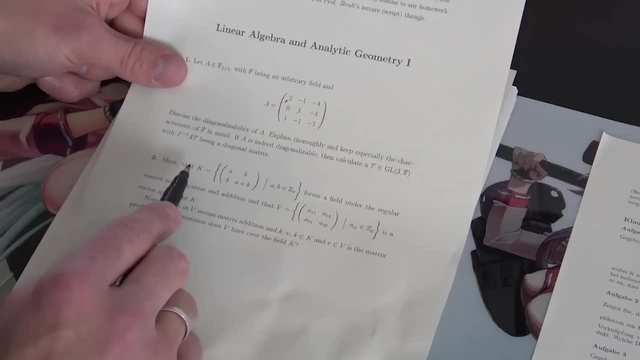 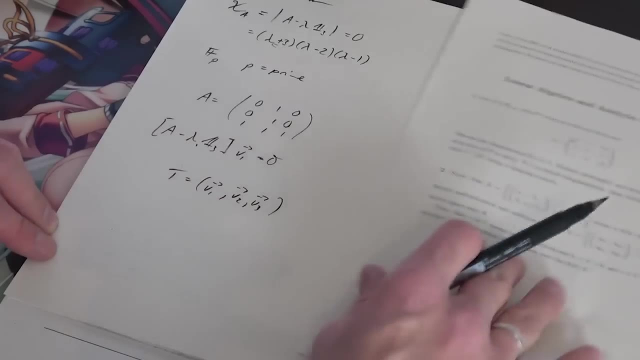 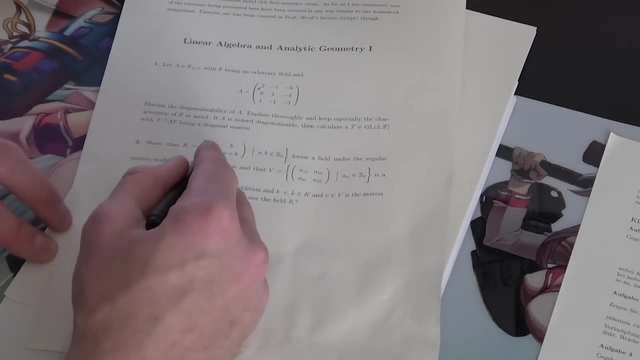 something. but there's actually an easier way. we can just go through all the elements in here in in k. what elements do we have in k? for example, in k we have um. let let a be equal to zero and b be equal to zero. then we have zero, zero, zero, zero, zero plus zero is zero if a is one and b is zero. 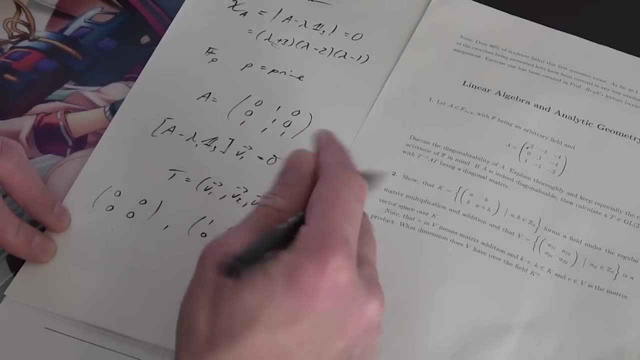 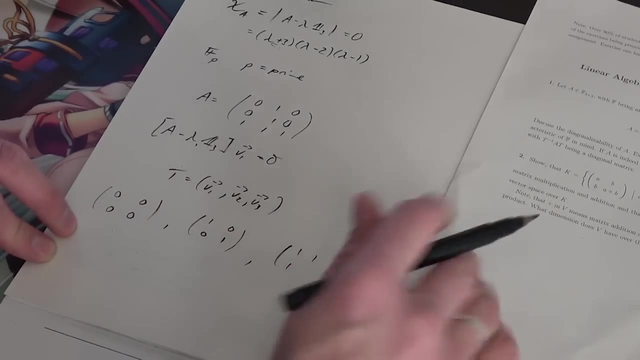 then we are going to get um, one, zero, zero, one plus zero is just one. then a and b are both equal to one. we are going to get one one one and one plus one is two, and modulo two is nothing but zero. and the last element that we are going to get 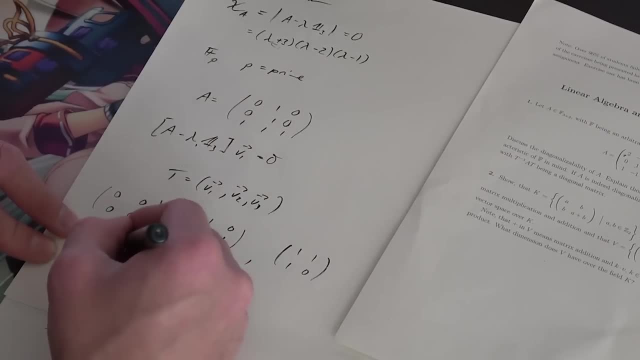 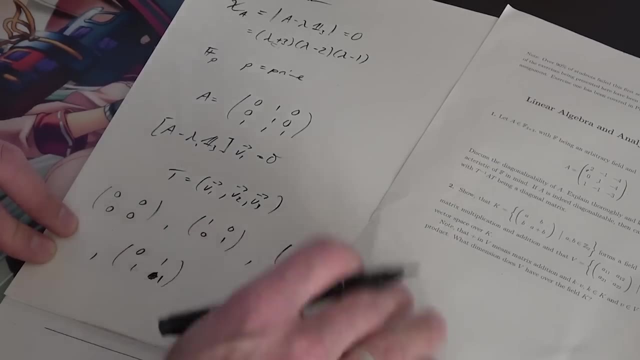 is when a is equal to zero and b is equal to one. so this gives us zero, one, one zero. those, oh, no one, i'm terribly sorry. those should be all the elements, four elements. you can do some combinatorics here also. v has four elements and b has one and b has zero. so this gives us zero, one, one zero. 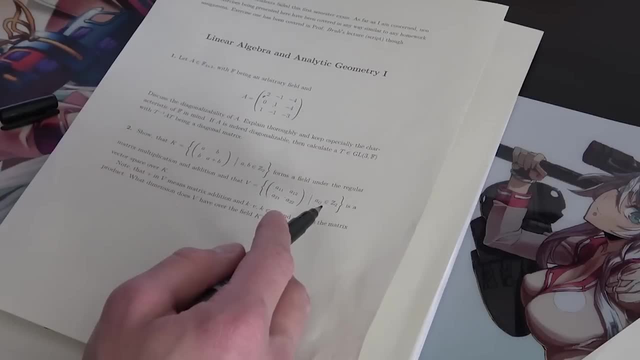 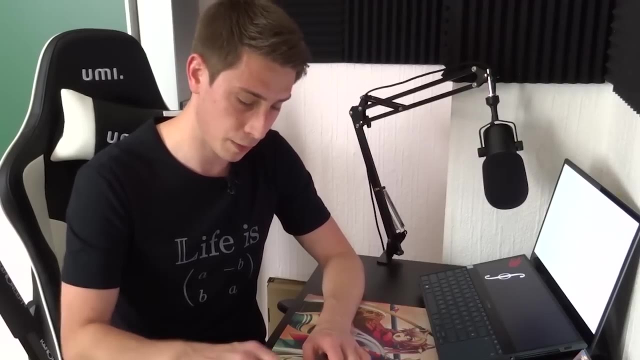 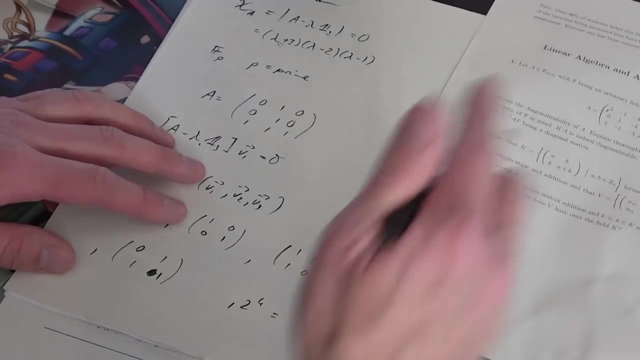 four distinct n entries and they are out of set two, so two possibilities for each slot makes two to the fourth power. two to the fourth power. yes, it's, it's. i'm terribly sorry it's going to be two to the fourth power. this means this is 16.. 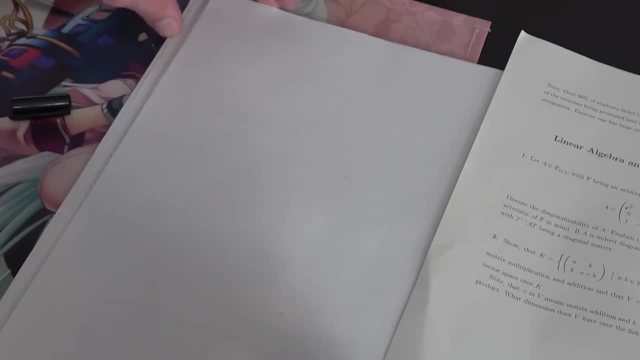 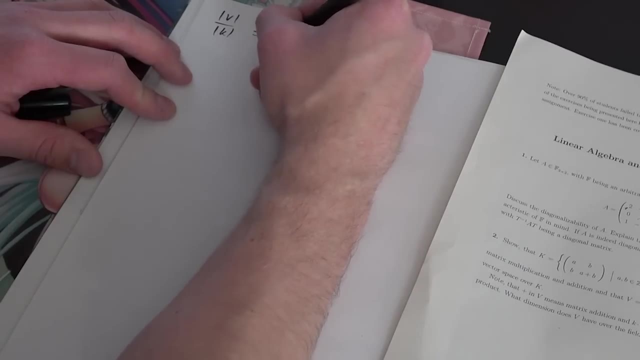 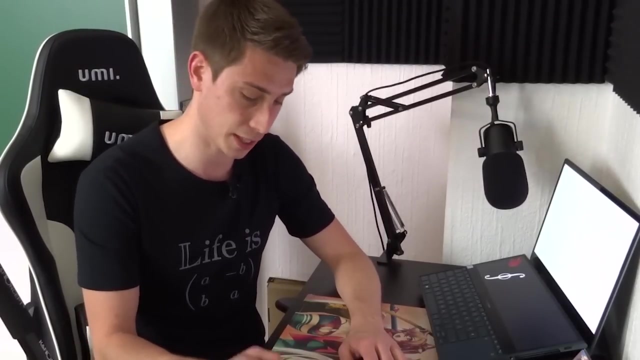 so meaning the dimension, the dimension of v over k is going to be 16 over 4, plus k is going to be 16 over 4 is going to be overall 4.. so this should work out. i hope this is correct. this was just my understanding, so you just can go through the. 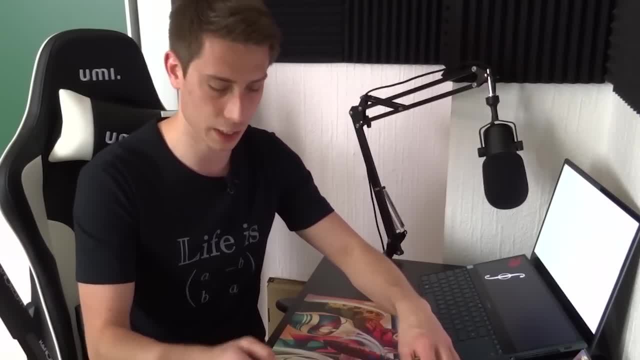 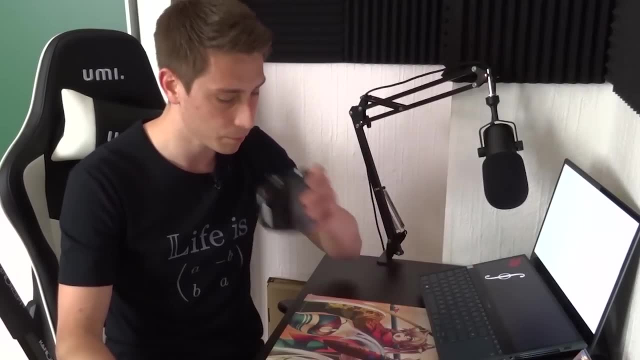 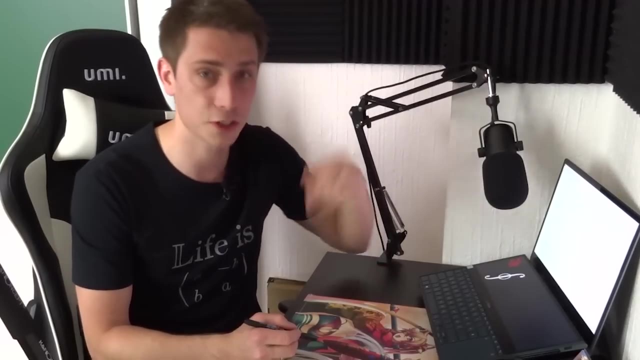 elements here, element wise- and this has been the second exercise- really easy too. just a lot of work. also for this exam, you have three hours of time, just as a little side note. now here comes the worst exercise in existence. seriously, this thing sucks so hard. it took me ages. 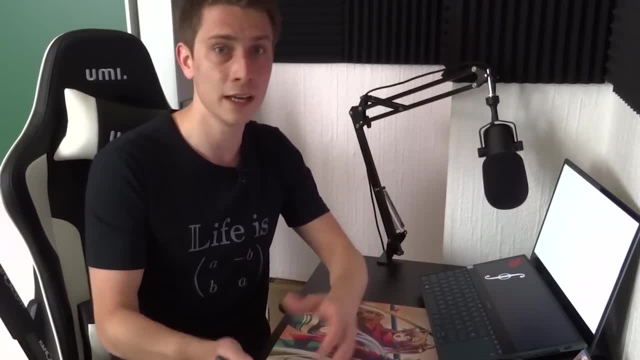 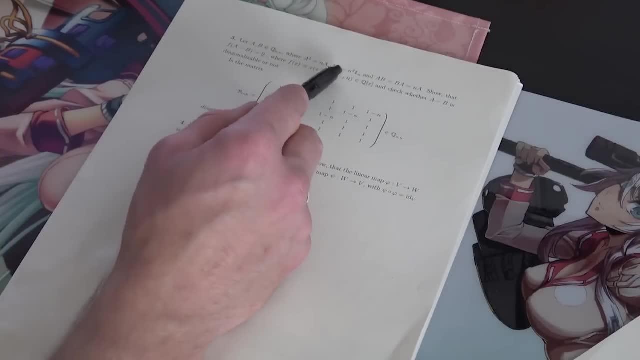 didn't know about a few theorems when it came to diagonalizability and minimal polynomials, So let a and b be element of q and n. where a squared is n times a, b squared is n squared times the identity matrix, n dimensions, and a- b is commutative. a b is b a and this is. 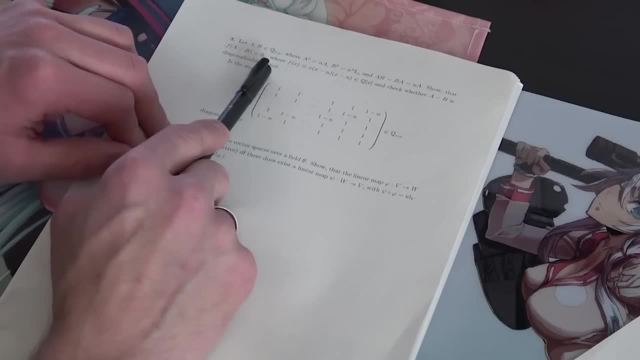 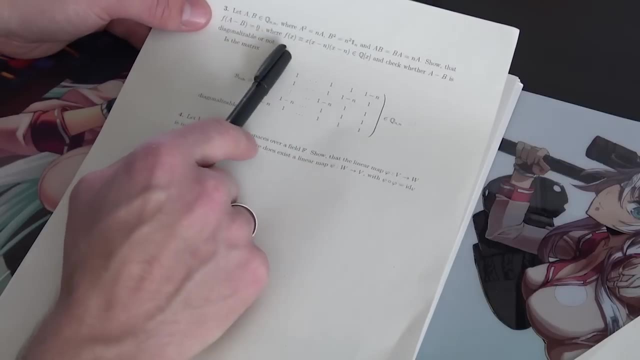 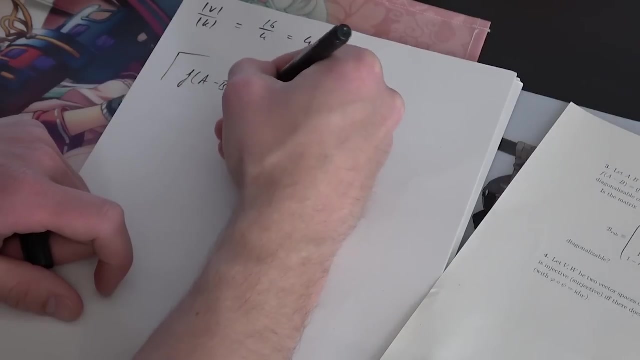 equal to n times a. We now need to show that f of a minus b is equal to the zero matrix. You just go through the calculations. You have f of x given. so that means if you plug it into f of x you are going to get f of a minus b is going to be a minus b times a minus. 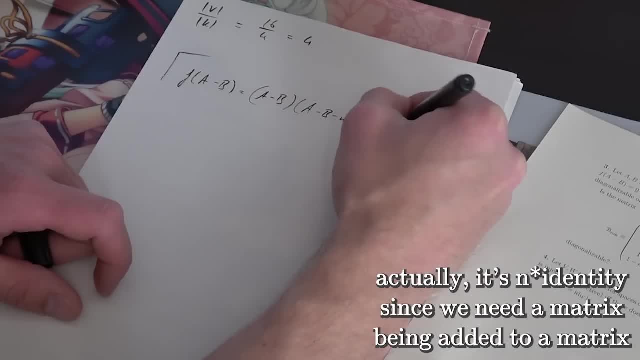 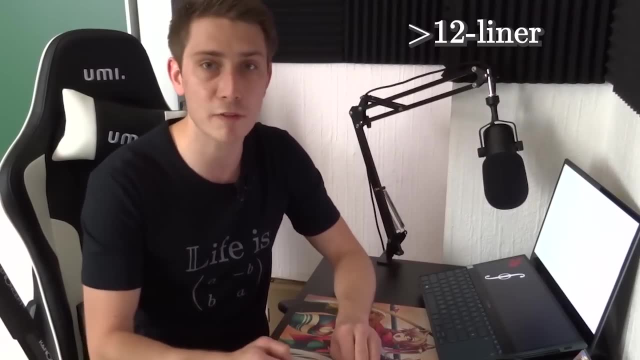 b minus n. times a minus b plus n. I'm terribly sorry. So this is just what it looks like and those are just calculations. It's an easy 12 liner, alright. So this is just really easy calculations. Nothing to really do here, just use the properties that. 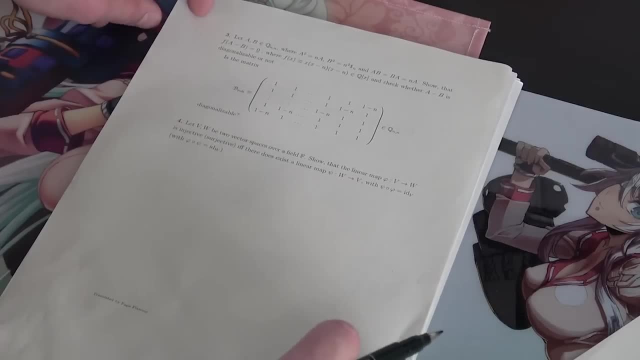 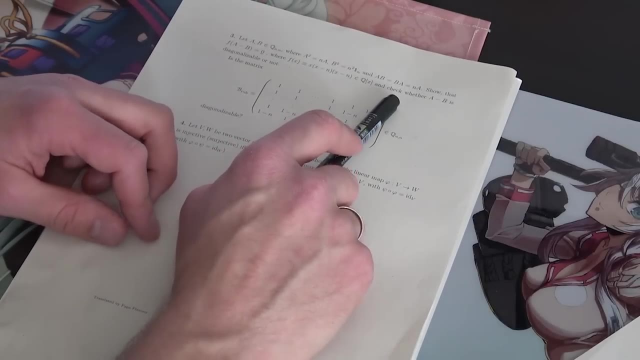 we have here. That's the easy part. You can get one or two points out of 12 from that. but now here comes the worst part, and we now need to check whether a minus b is diagonalizable or not. If you have the theorems at hand, it's not going to be a problem, but if you don't have the theorems, 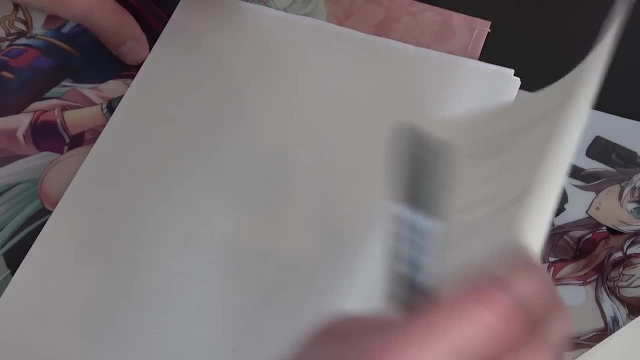 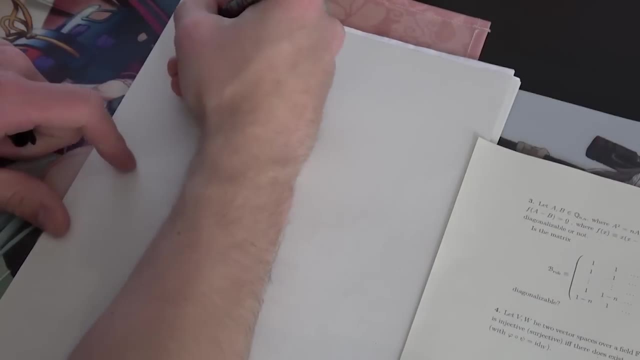 at hand, it's going to be extremely problematic. So the first one is we have that f of some matrix m, so a minus b is just some matrix m. If we have f of a matrix m being equal to the zero matrix, then this implies that the minimal polynomial in this matrix m is: 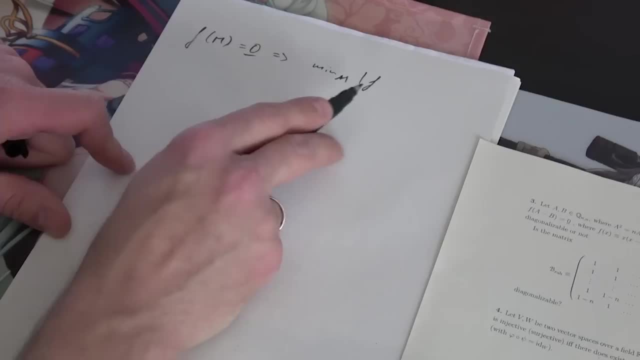 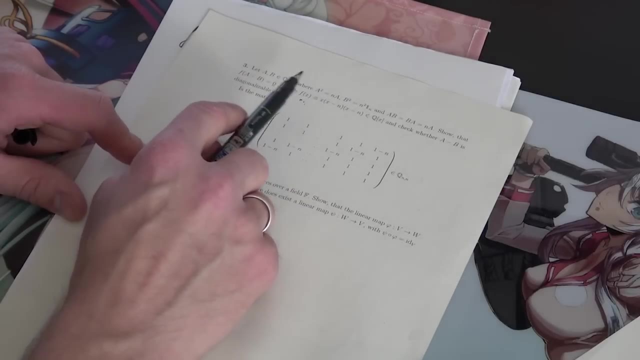 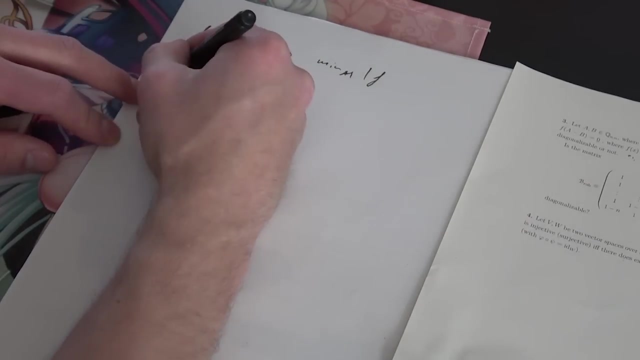 going to be dividing some f, for example, So this f being this one right here. So we don't know if this thing is actually the minimal polynomial, but yeah, it could be smaller, but that's really not the point here. If we have this, then a matrix, that's another theorem. 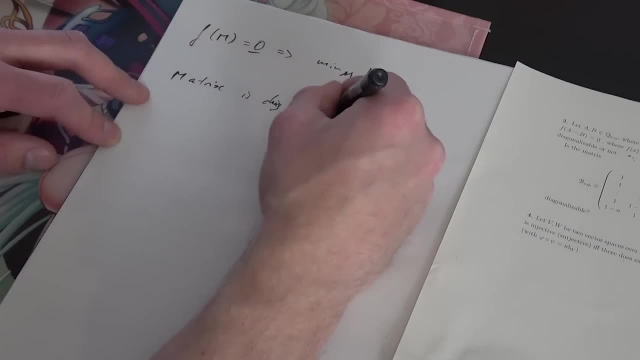 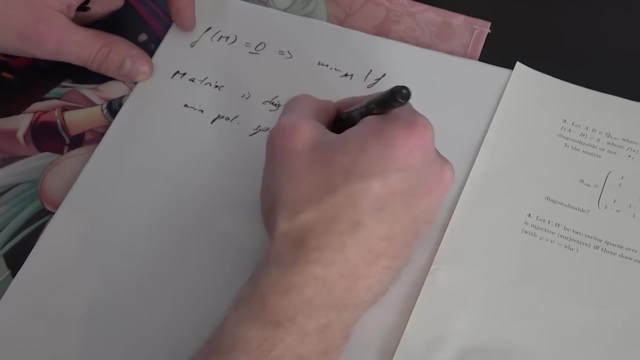 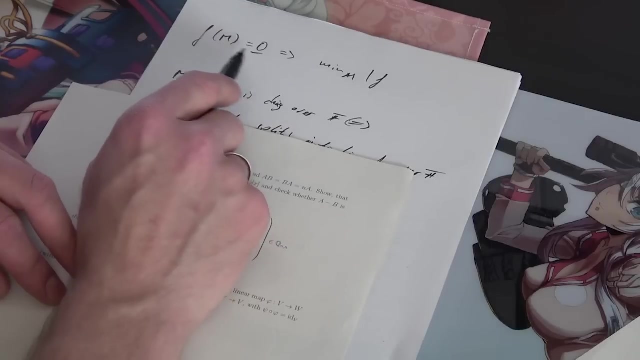 a matrix is diagonalizable over some theorem Field f. if, and only if. so that's an equivalence. the minimal polynomial splits into linear factors over this field. So this is basically what this theorem says. So our f of m is equal to the zero matrix. This implies that the minimal polynomial divides f, but this also 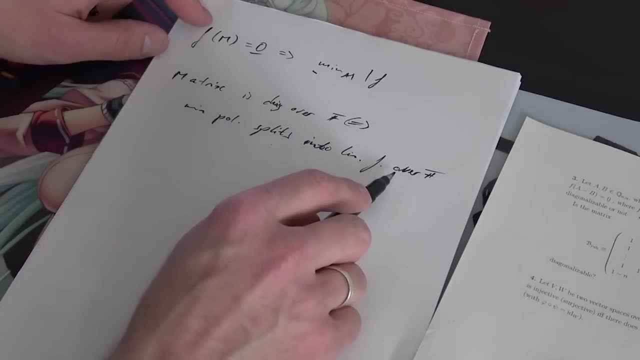 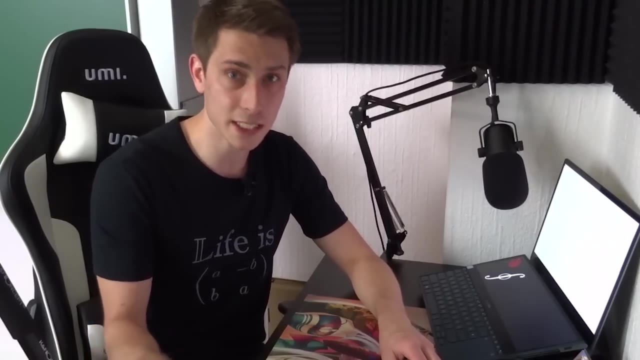 implies that our minimal polynomial splits into linear factors, and this is equivalent to the statement that the matrix is diagonalizable over this field. It's some kind of theorem, I didn't know that. Cedric Brendel helped me with this, so thank you, Cedric very much. I didn't know about this. 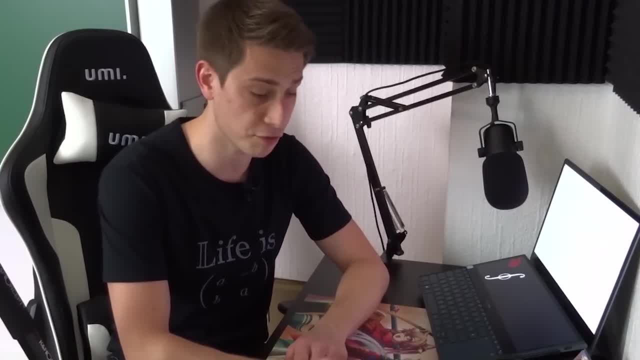 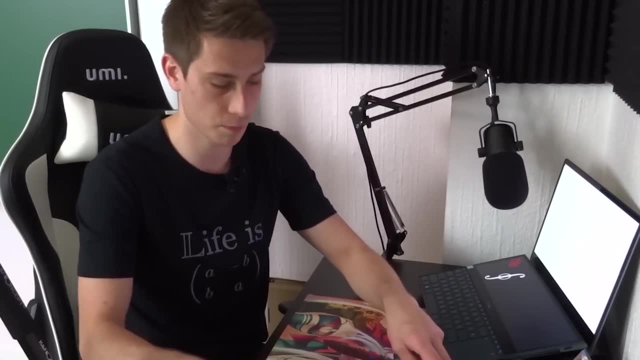 theorem and, yeah, I would have been seriously fucked in this exercise when I would have had it in the first semester. So I really wouldn't know about this theorem. probably, Even though I went to the lectures, I wouldn't know about this and probably this and the 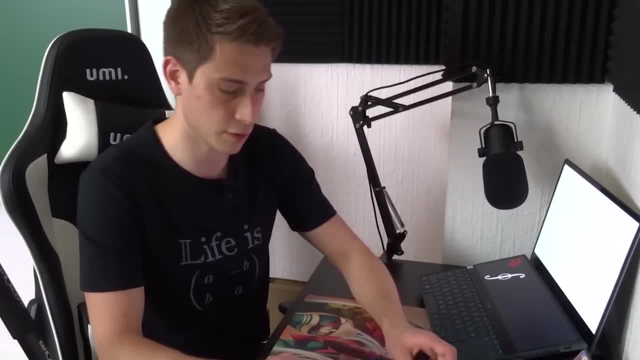 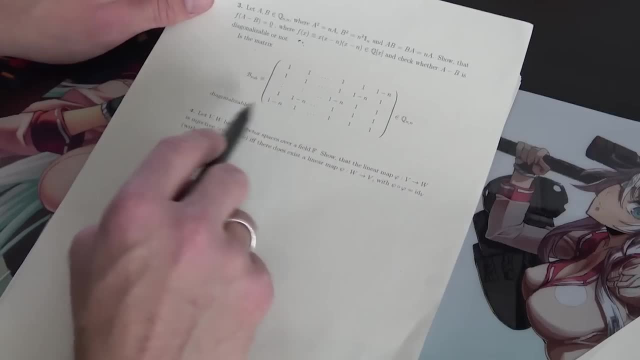 last exercise are the whole reason why so many people fail this thing. Next is the matrix: blah, blah, blah. I called it b Index, ra, Ra, Ra, Diagonalizable, And this thing is absolutely ingenious. this last part, It's really ingenious. 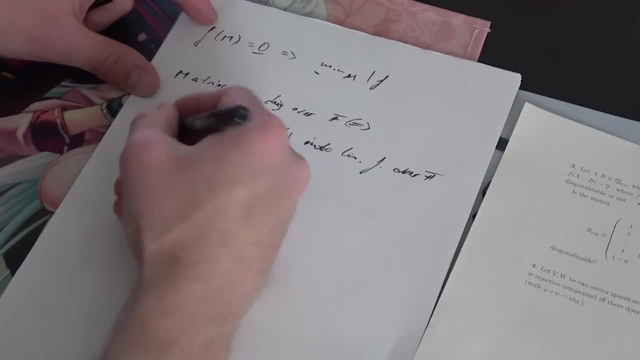 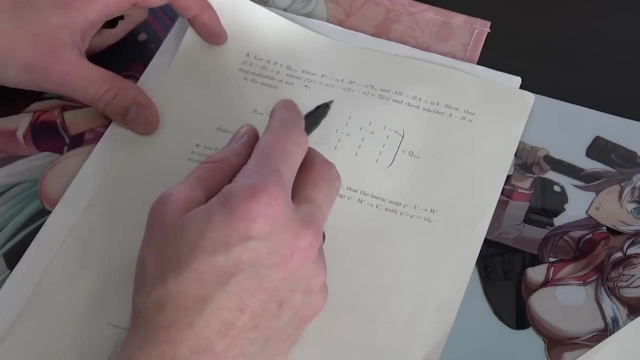 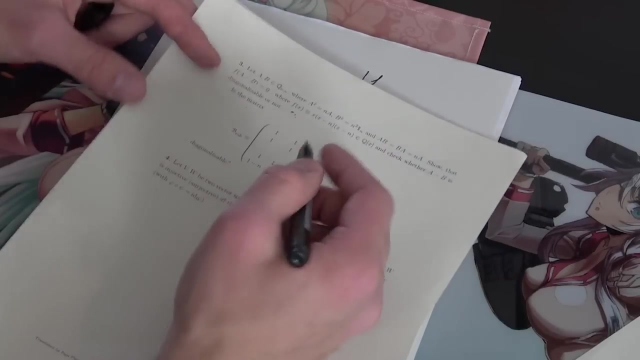 If you take a look at this matrix, we know that our b is nothing but well, what do we have? This is just a whole bunch of ones. So this is just a matrix in n dimensions with ones everywhere minus well, a matrix with n's on the nut main diagonal. 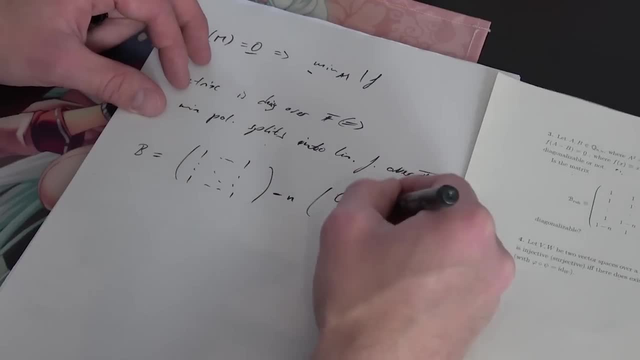 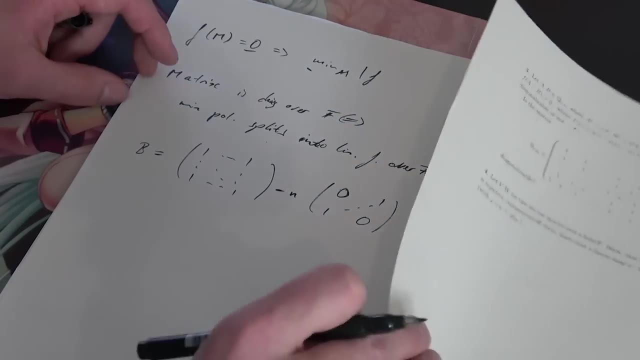 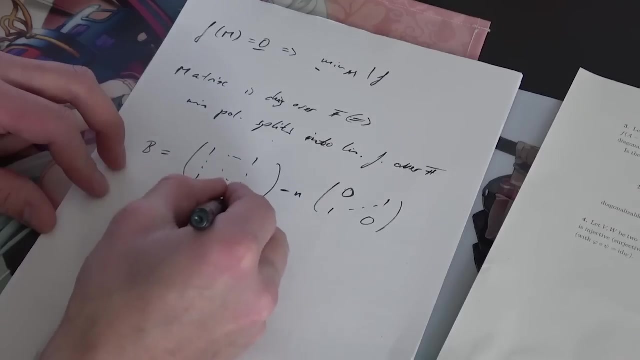 Okay, Minus n times a matrix where we have zeros everywhere except for the nut main diagonal. This is really similar to the exercise we had on the algebra and arithmetic one. Now, if we just check for some properties here, Let us bring it back to f. 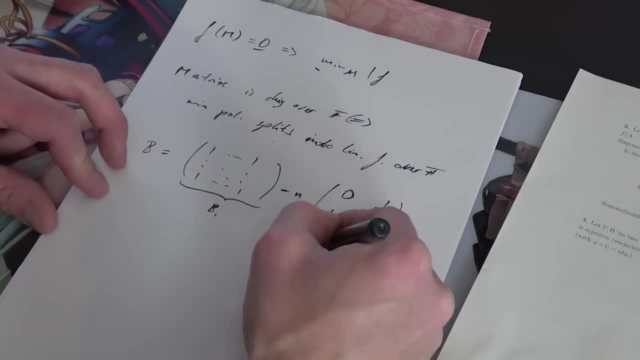 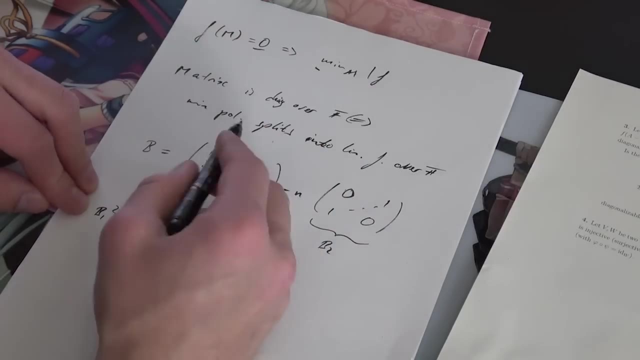 Let's call this thing b1 and this thing right here is b2.. Okay, then we have that b1. squared is going to be: if we square this, we are going to put this on front- Then we have, in the first spot, One plus one plus one n times. 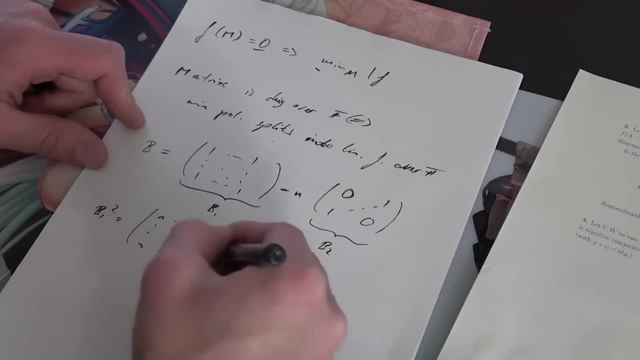 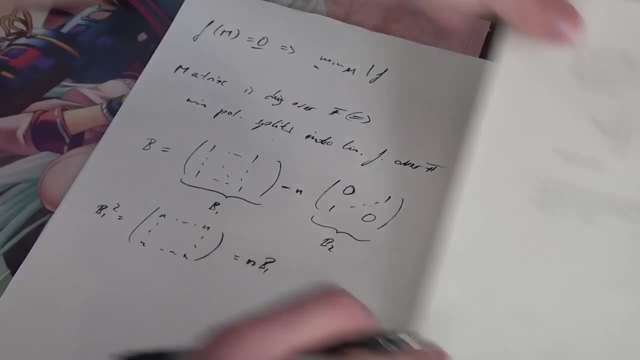 This is just going to be n, n, and we are going to have n everywhere. Meaning overall, this is n times b1.. N times b1.. Hmm, This kind of rings a bell We had a squared, is equal to n times a. 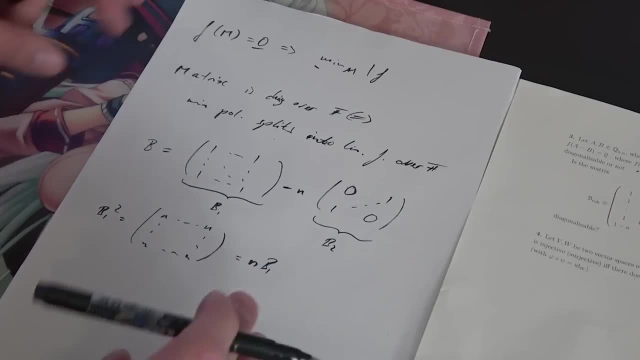 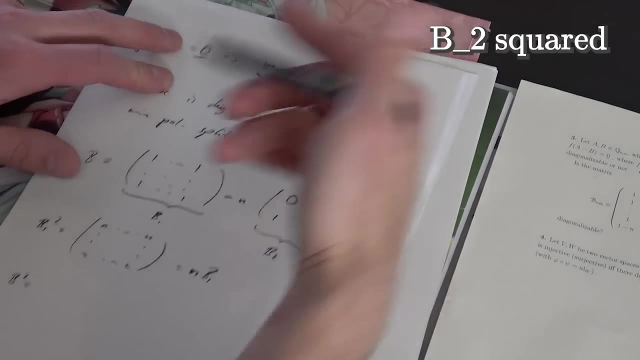 Now we have: b squared is equal to n times b. Oh, that's absolutely ingenious. And now for b squared. we have that b squared is nothing, But if we put it on here, one one and everywhere, zeros on the other places, meaning this is: 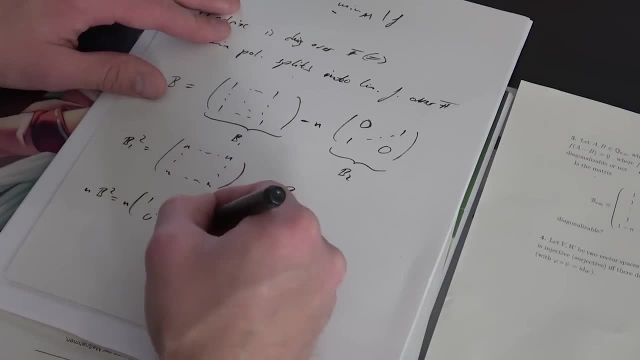 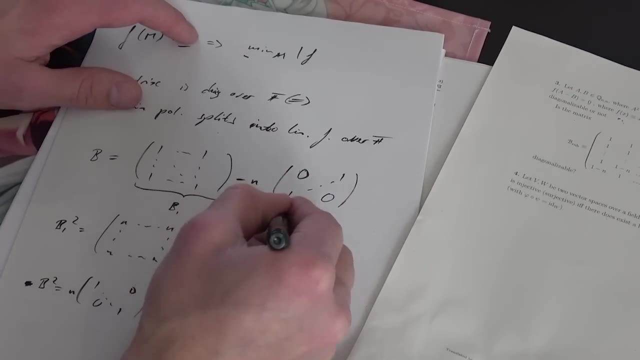 just the identity matrix. If we put an n to the front, it's going to be n times the identity matrix overall. Yes, if you include the n in b2, then it's just going to be n squared times the identity matrix. 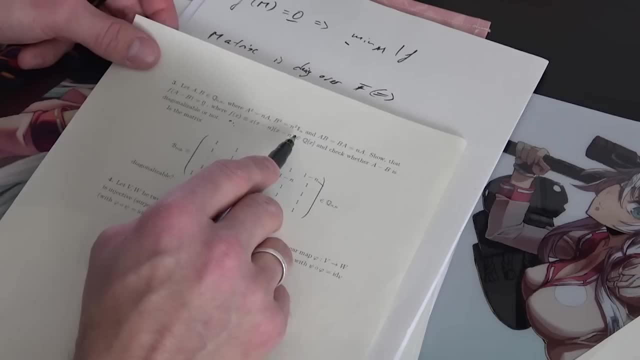 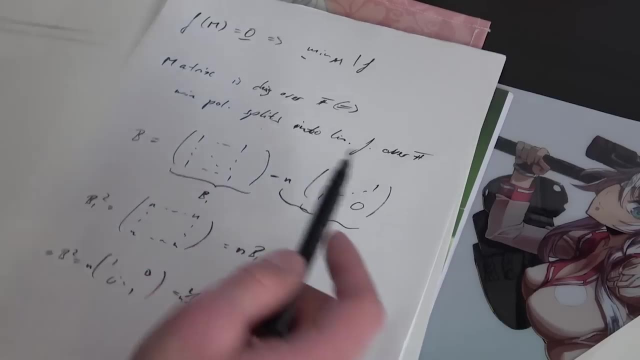 Let's put it like this: This is just the same as b squared being equal to n squared times the identity matrix, meaning overall. Those matrices that we have defined here basically go by the rules of a and b up here. Then we do subtract b1 from b2.. 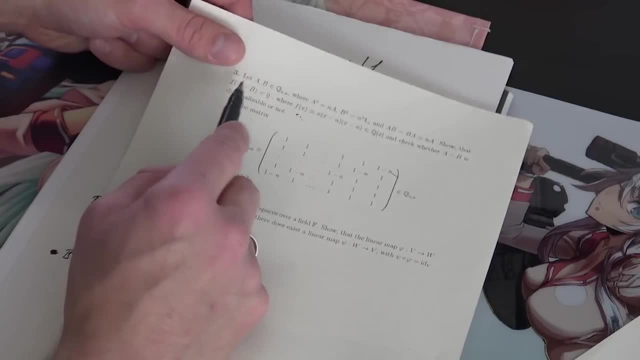 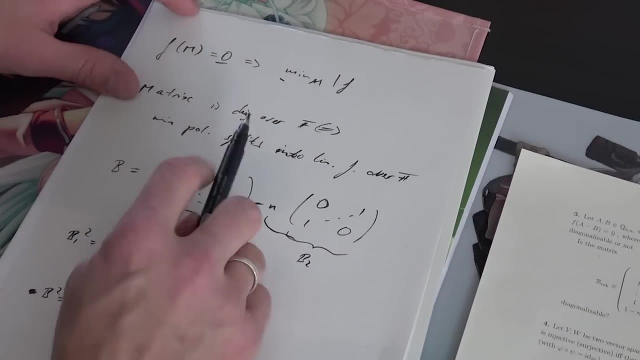 This is just a minus b, basically, And f of a minus b is going to be equal to the zero matrix, And we know that it's going to be diagonalizable by this piece of shit that we have here, And then we are done. 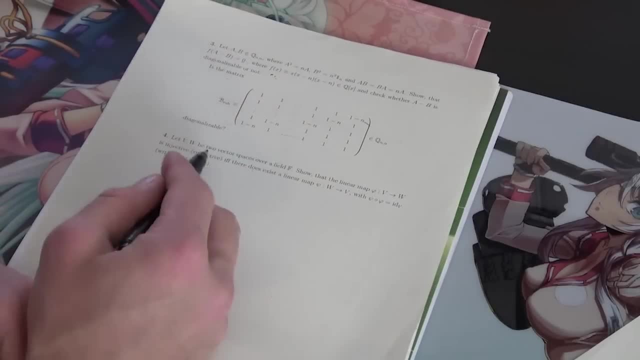 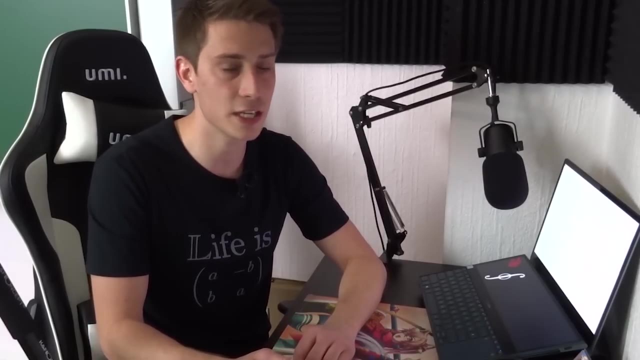 And now for the last exercise. I'm not going to go into too much detail about this. This is just a standard surjectivity matrix. Okay, It's a linear algebra lecture note that you are going to find in each and every linear algebra lecture note out there. 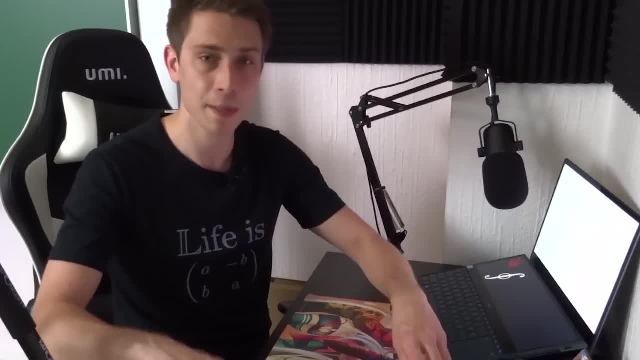 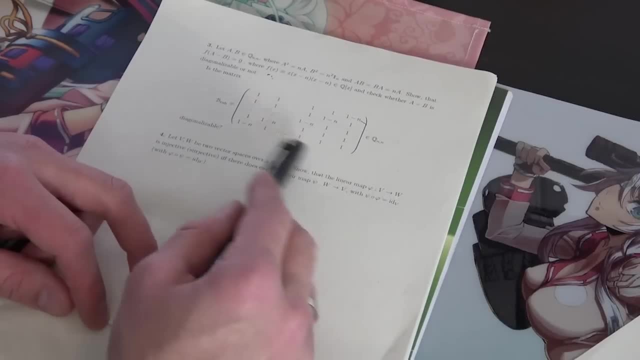 And you are going to have a ton of solutions out there on MathStack Exchange. Only one or two words about this. This result in linear algebra is extremely important because it basically just says overall that if it's bijective, for example, that we can express each and every linear transformation. 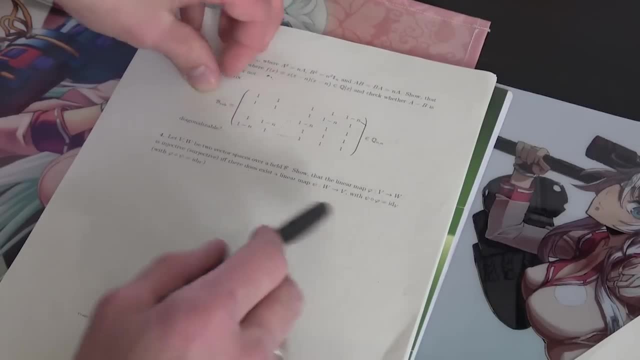 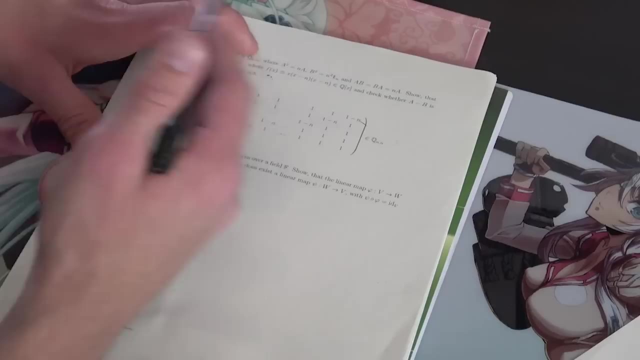 as a matrix if it's finite dimensional. This is just a really big, important result here And it also says something. It says something about those linear transformations, For example. if you want it to be bijective, then it needs to be a square matrix, for example. 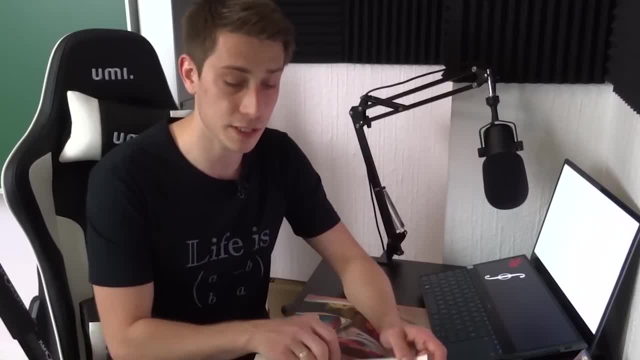 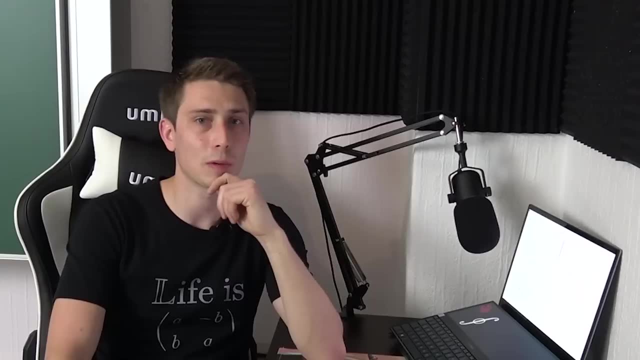 So this one is really important Now. we went through this exam and now a few last words. So we went over this exam and now, once again, we would like to talk about the reasons why so many people failed, And I believe it's kind of clear why so many people failed. 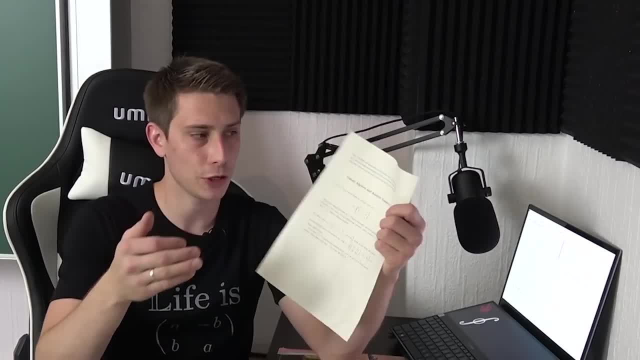 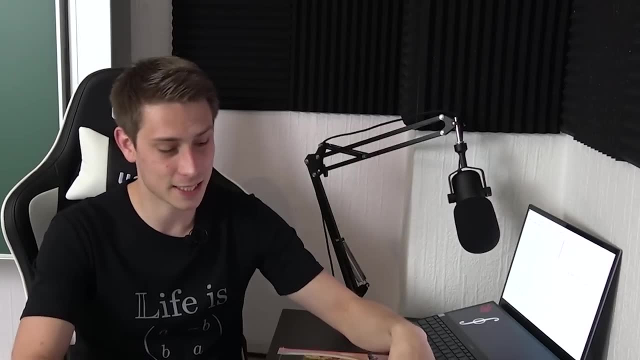 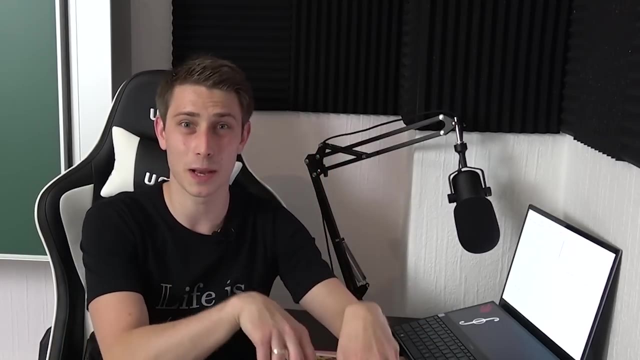 So we had those first few lines where a student said from her experience that none of this really has been covered by professor in any way. And yeah, this is kind of the worst thing. So if you get only really rigorous and never practice all this stuff that you need to apply, 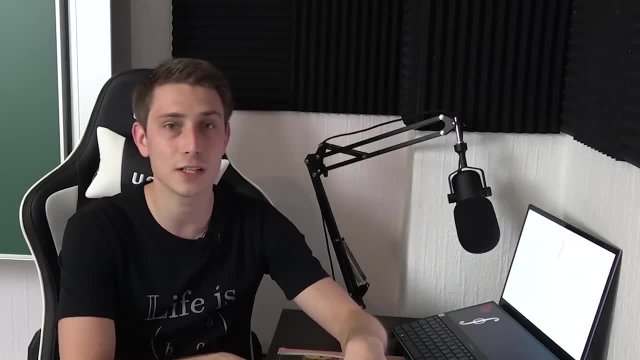 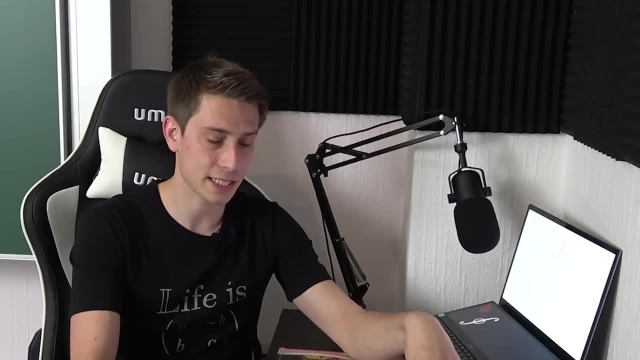 here in those exams, then you are pretty much rigged, So there's no way around it. This is probably by far the greatest factor why this happened. Also, in a normal case in linear algebra in the first semester, students won't get. 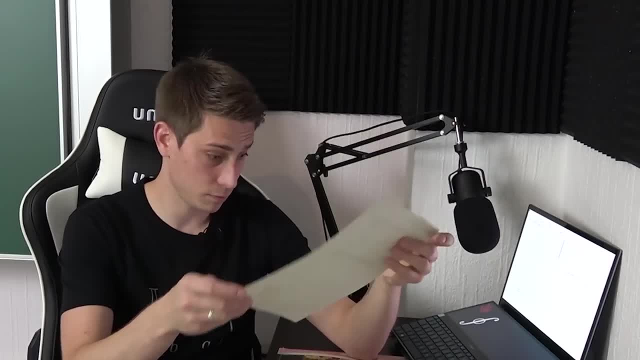 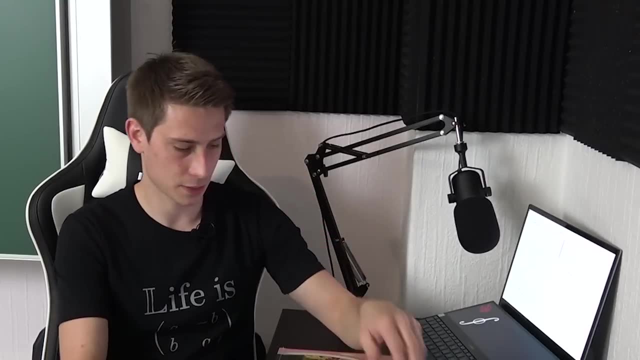 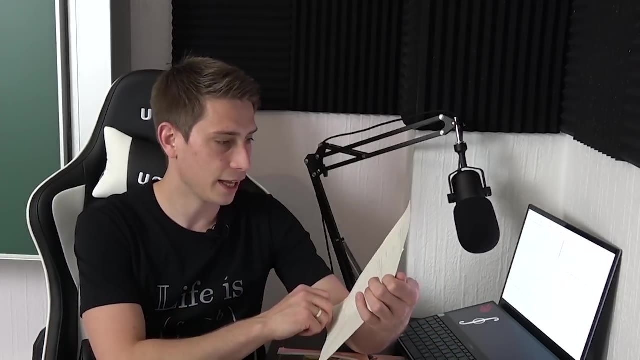 any real rigorous proofs That they need to be, That they need to do So. as for the linear algebra courses I visited, there wasn't really any rigorous proof that you need to do, And I know from my experience that a lot of people struggle with search activity and injectivity. 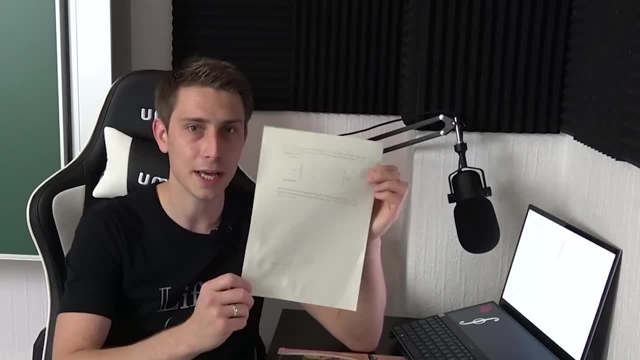 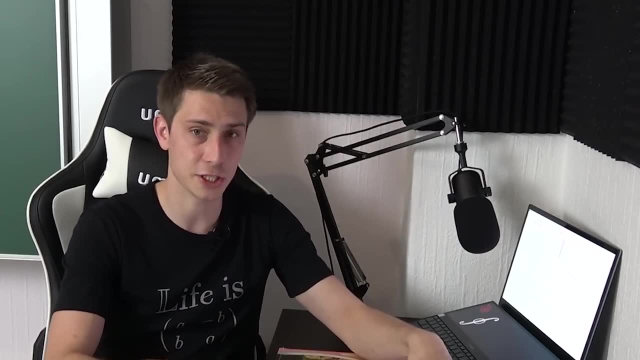 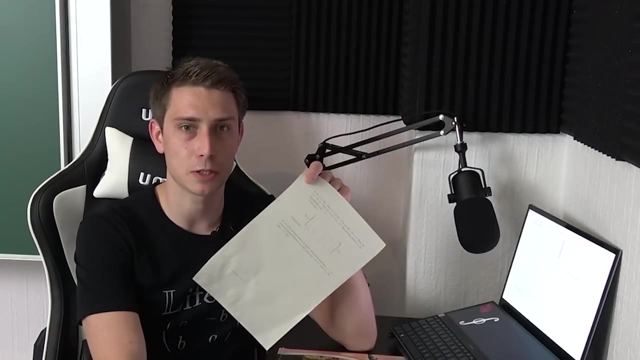 And yeah, many people suffer from not being able to pull off proofs in the first semester, Me included. I couldn't do proofs in the first semester. Took me ages to get some proofs done. Alright. So yeah, other than that, third exercise is just an absolute killer. 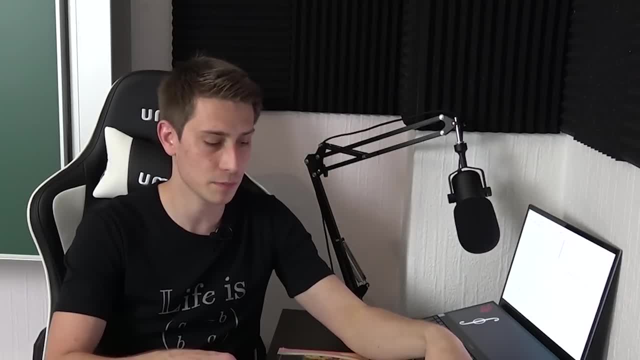 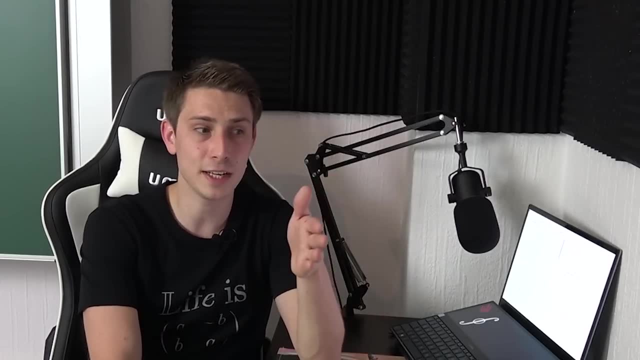 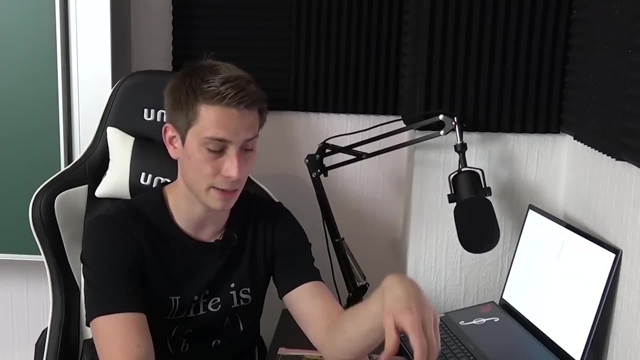 This thing is so annoying, and if you don't know about the theorems that I have presented here, then you are also pretty darned, And that's the thing that also happened to the last exam I have presented to you guys. So the algebra and arithmetic exam. 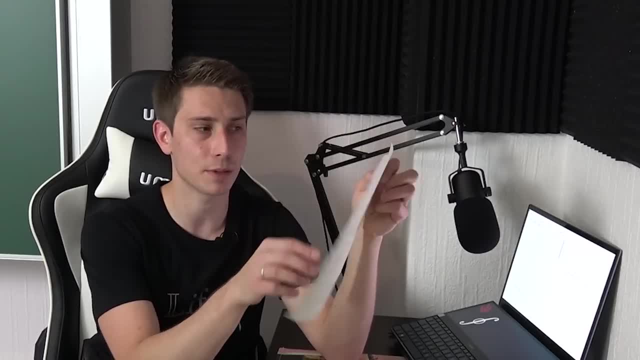 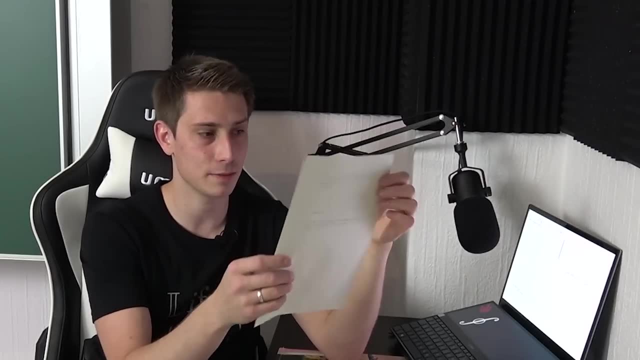 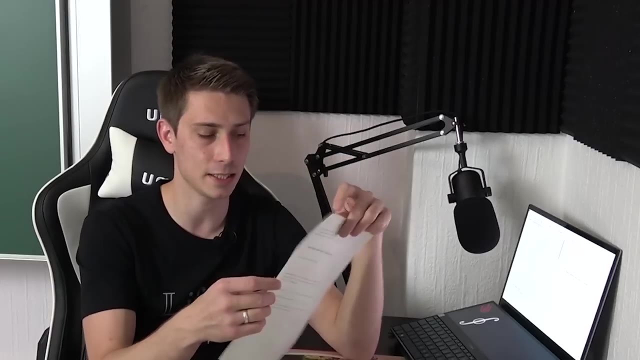 We had that the first two exercises were doable. but the last two exercises weren't really doable for most students And those get you half of the points and getting a perfect score on those two is already kind of hard for most students. So if you do one little mistake here and you can't really get any points here, then you